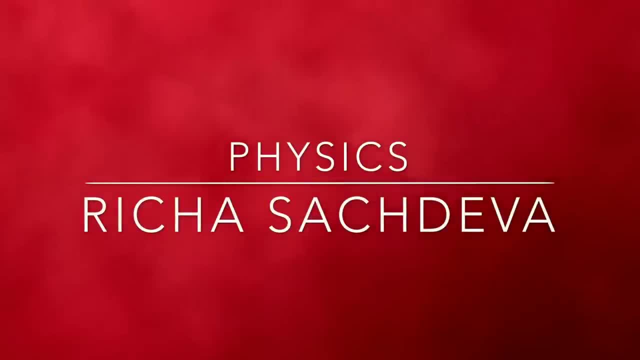 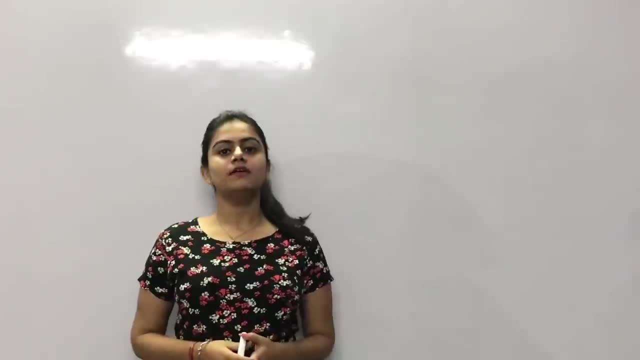 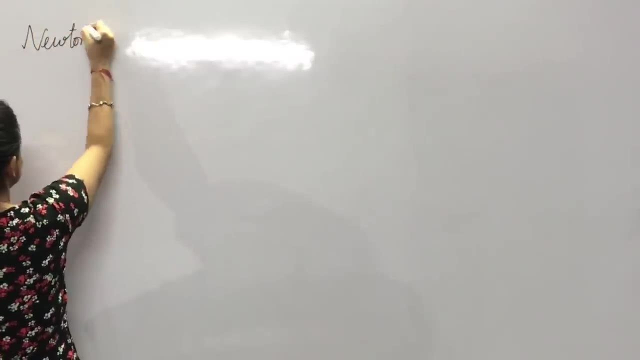 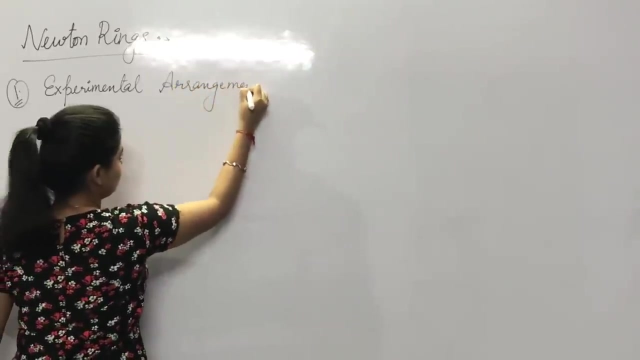 Hello everyone, my name is Richa Sachdeva and today we will start wave optics. So in wave optics, our first topic is neutral rings. So for neutral rings, we will firstly study its experimental arrangement, Or we can say construction. So for its construction, we 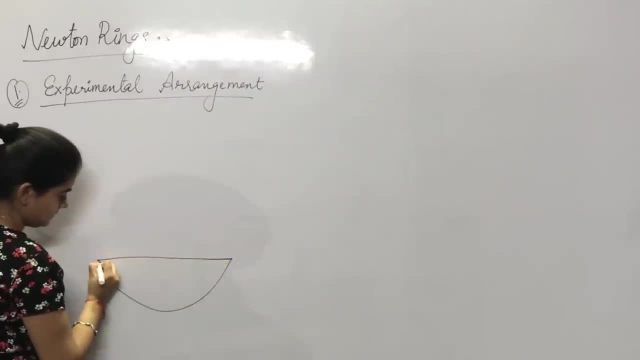 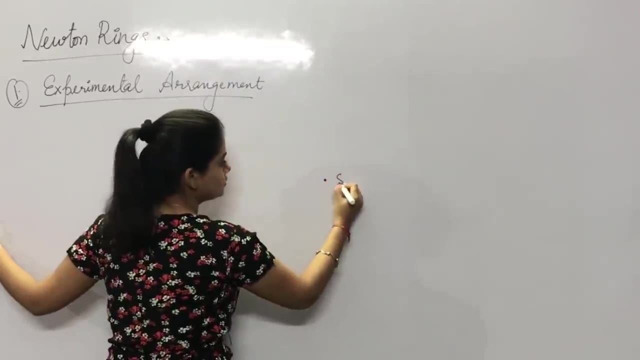 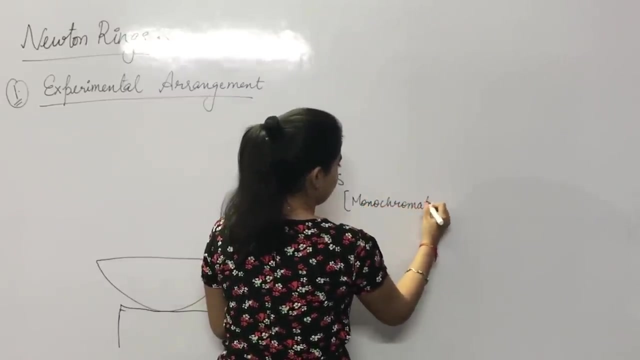 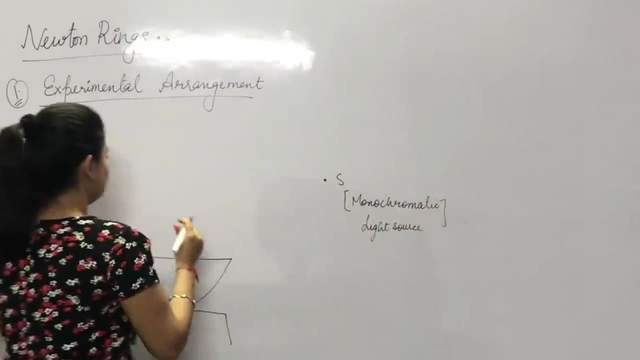 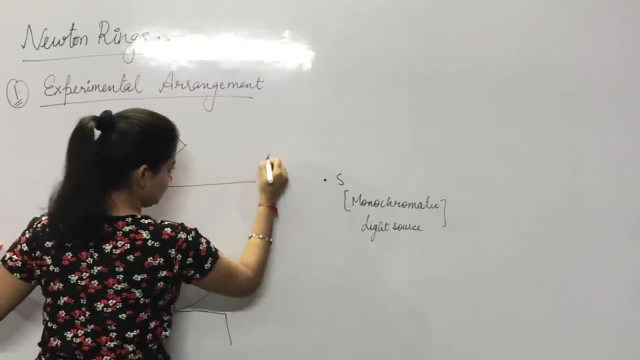 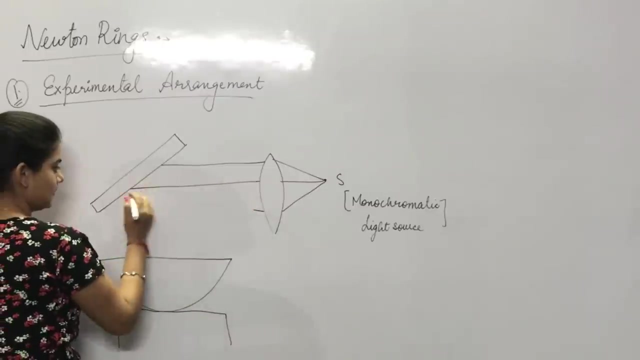 will take one plano convex lens and we will place one plain glass plate below this. We will take one monochromatic light source And then we will place one more glass plate at 45 degree angle from the axis- principal axis- of this convex lens, So the rays will start coming from this source and they will 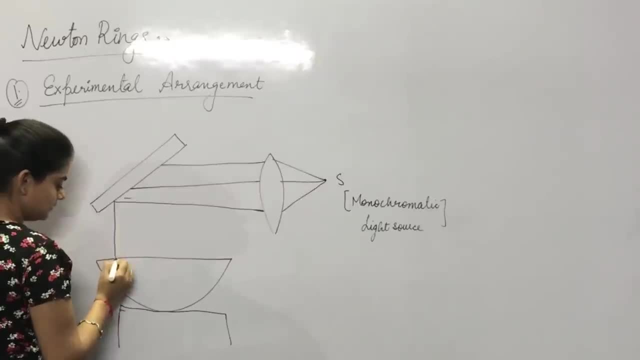 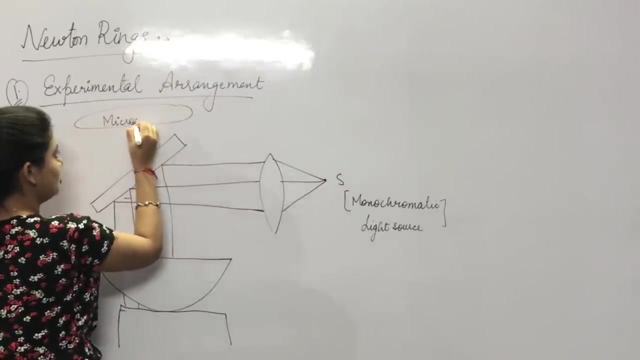 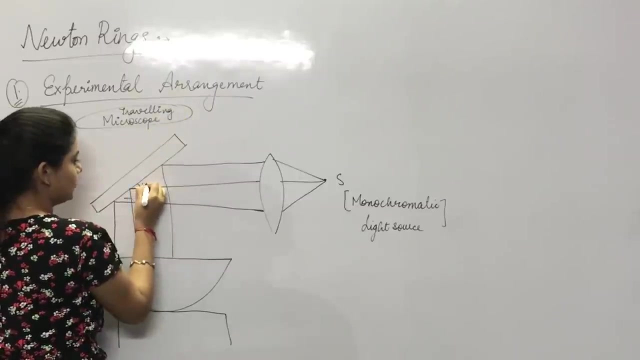 be imposed on this glass plate. Okay, Now we will take one�� one, And here we have one microscope. This is a travelling microscope, so we can adjust it according to our requirement. This is at an angle 45 degree, So this is a monochromatic. 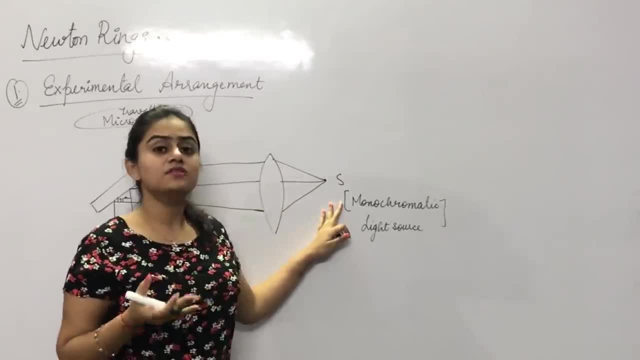 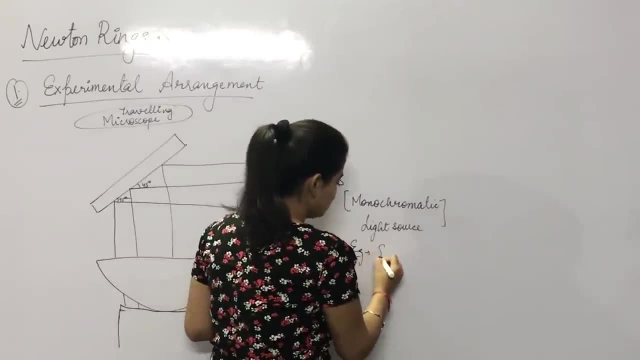 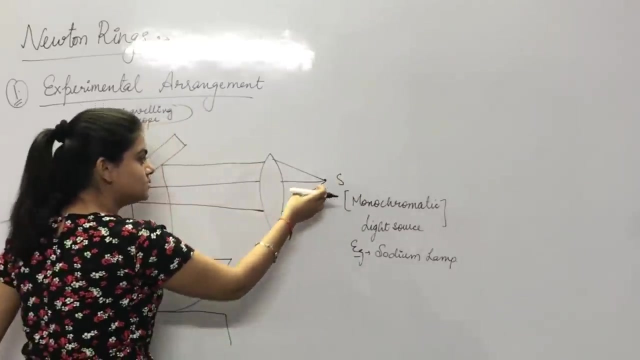 light source. What does monochromatic means? It means we have a sodium lamp or any light source which just emits one type of light, Right of wavelength. So we can see, example, sodium lamp. So light will start coming from this. 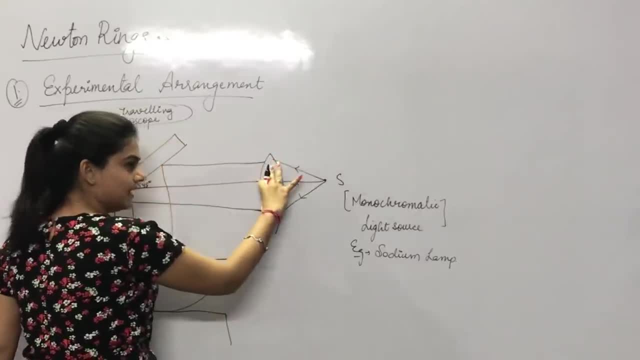 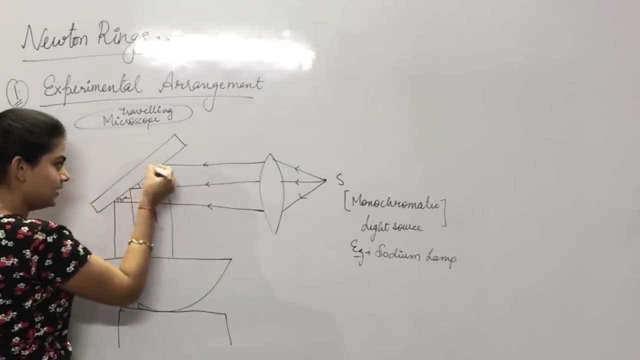 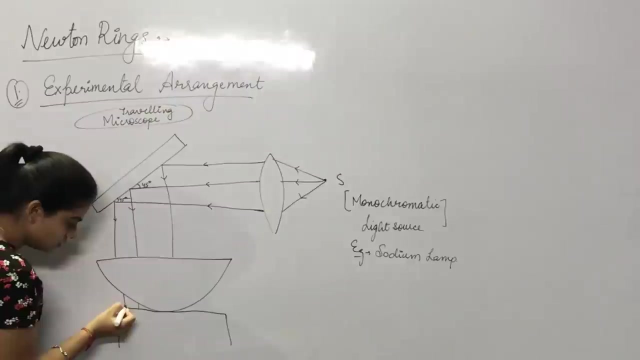 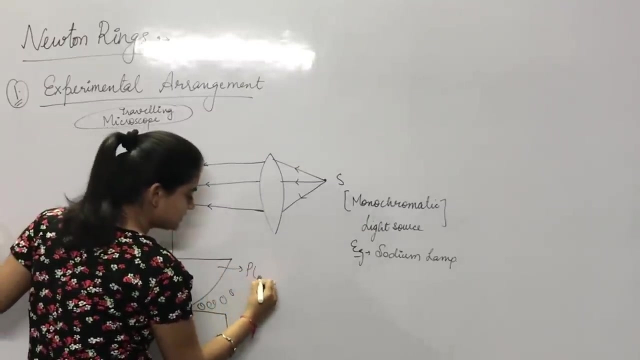 source. It will fall upon this lens and then it will proceed towards the plain glass plate which is placed at an angle of 45 degree. Then it will reflect. from this, It will go down and then it will go through this area. Here we have an air film form. This is a planoconvex. 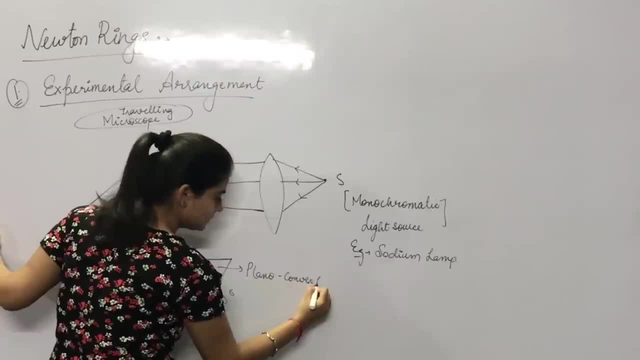 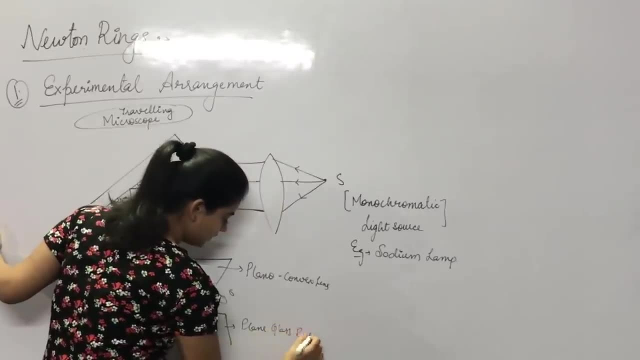 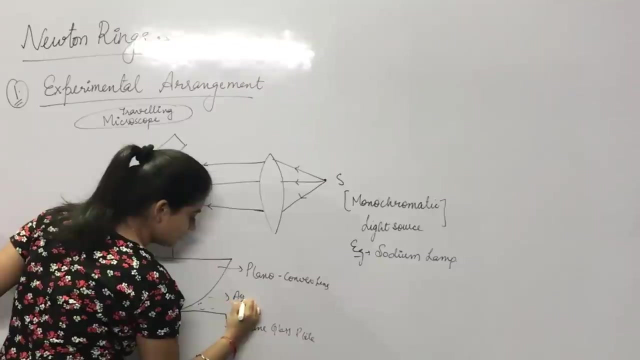 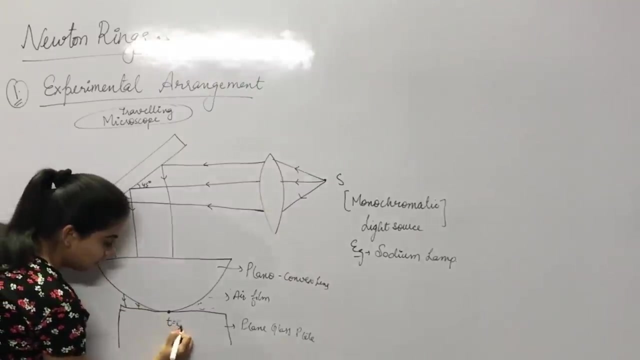 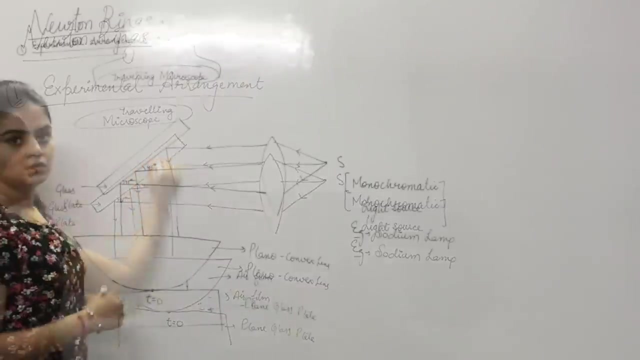 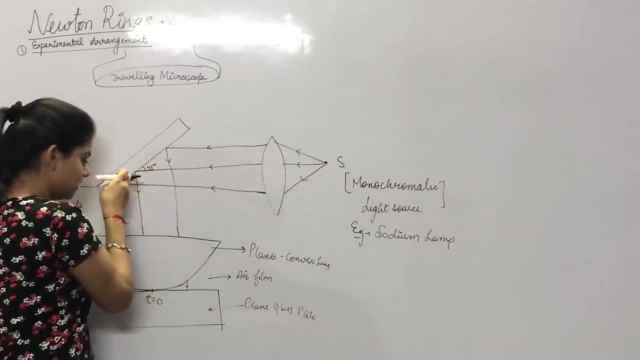 lens. This is a plain glass plate. In between these we have an air film form Air film. So the thickness of the air film is T is equal to 0.. This is again a glass plate, So the light rays coming from this source will travel like. It will take this path first, Then it. 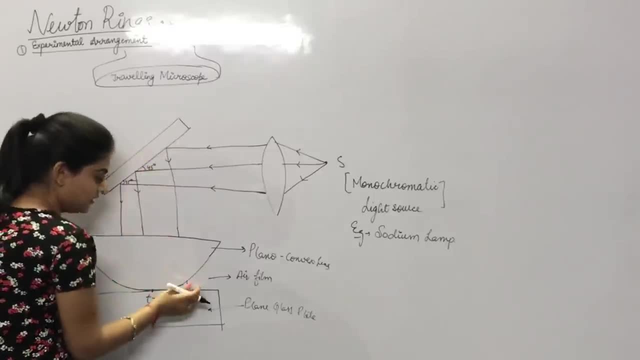 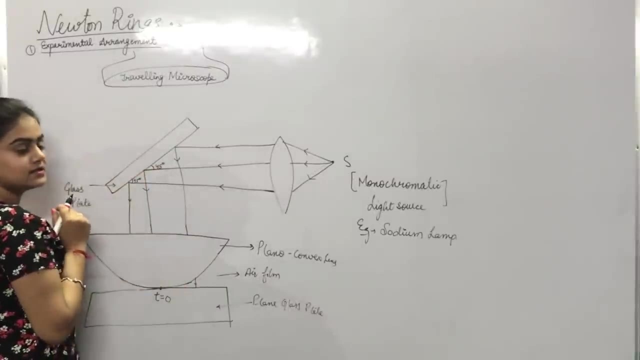 will go down due to the reflection from this glass plate. Then here an air film is there. Here we have an air film formed Here. the thickness of the air film is T is equal to 0. So as we move from outside that the thickness of the air film increases. Then the air film 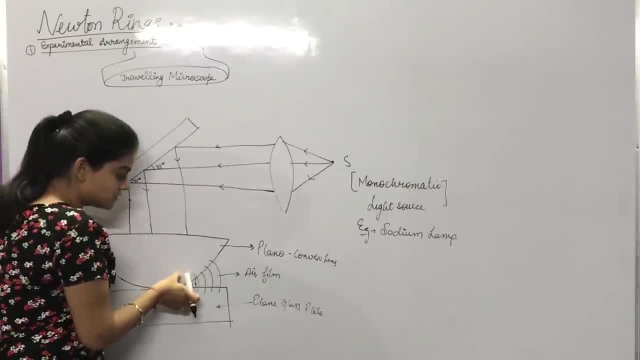 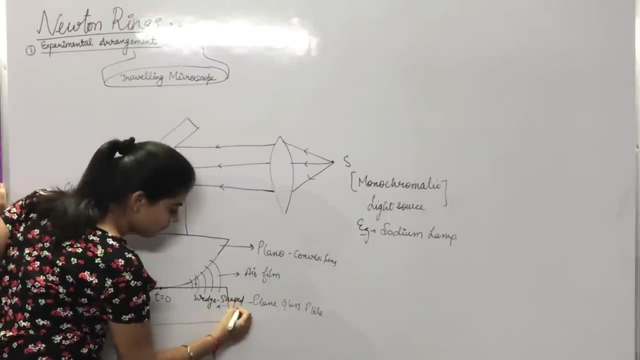 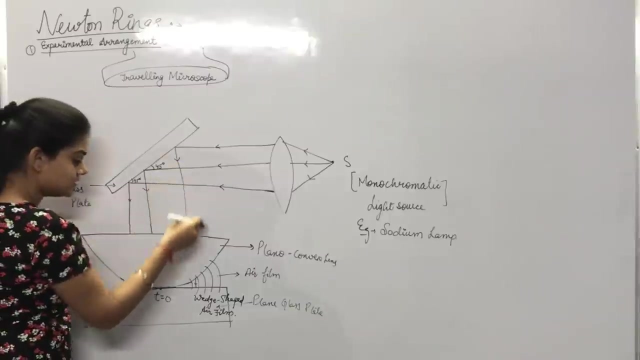 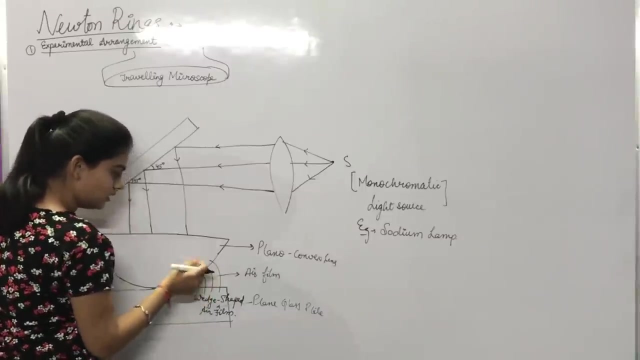 whose thickness is increasing gradually. it is called as veggie shaped air film. Veggie shaped Air film Right Reflecting from here. it will reflect back some part of this From this part of this glass plate. So it will reflect back. look here. So that is skimmed. 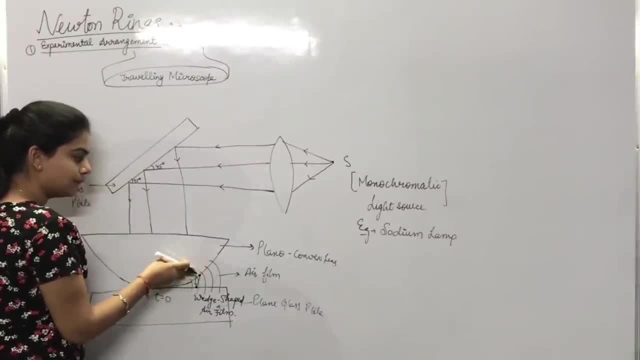 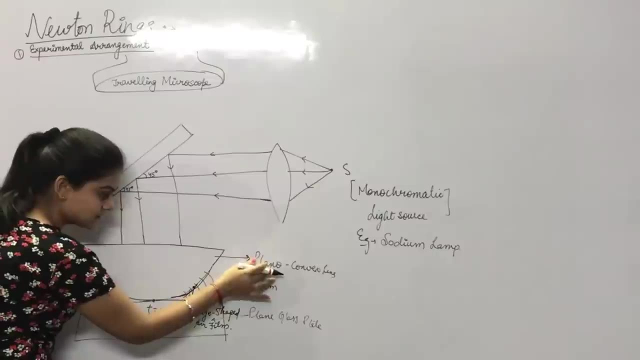 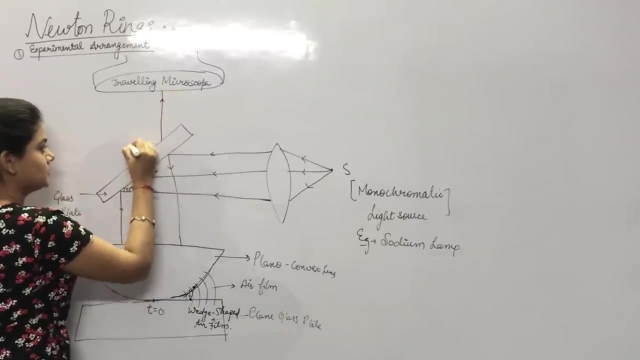 And some part will reflect back from the bottom part of the plano convex lens, Because air film is nothing but the distance between bottom surface of plano convex lens and upper surface of plain glass plate. So we will send the light back after travelling from here. 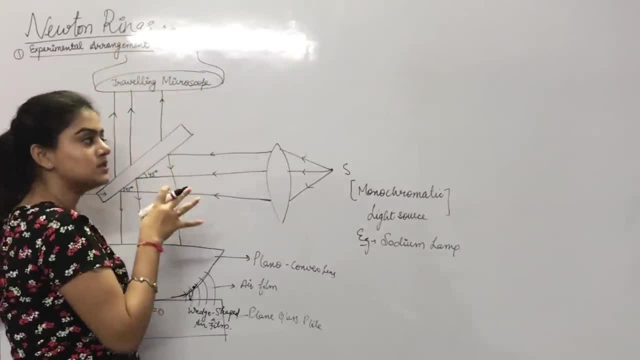 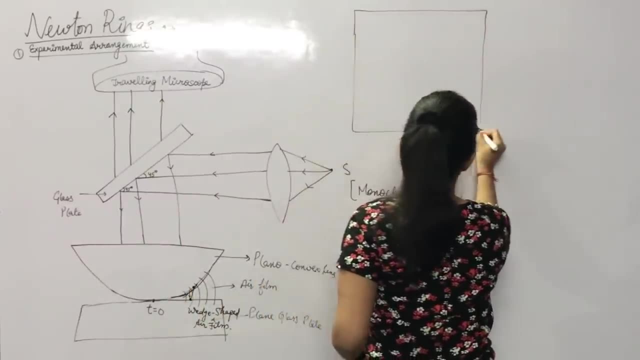 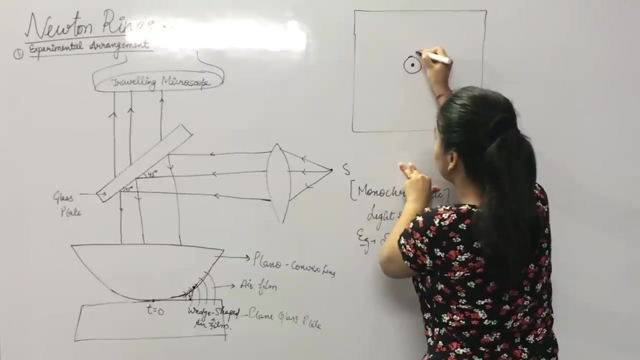 So what we will see in the eye piece of the microscope will be something like this: So let us suppose this is the eye piece of microscope. In the eye piece of microscope we will get something like this: We will get the central fringe dark, then we will get one bright fringe, then dark fringe, then bright fringe. 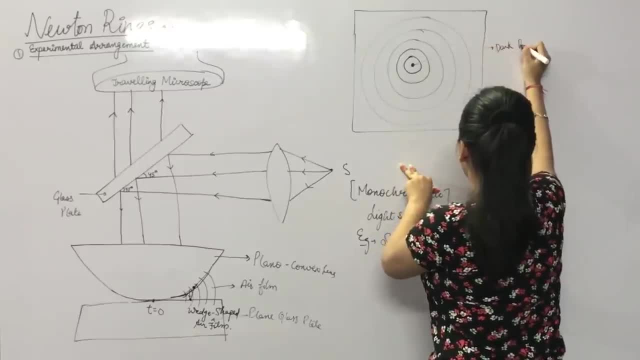 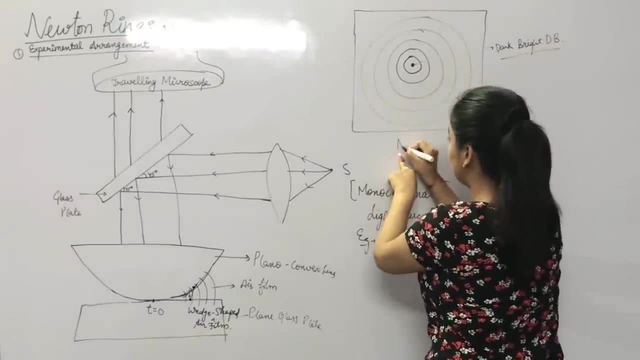 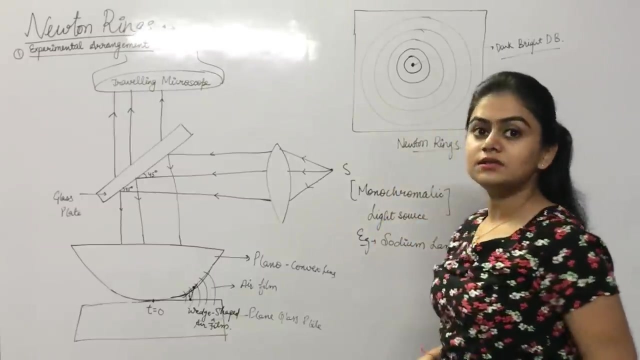 It will start from dark then bright, then dark, then bright, Like this, Like this. So we will get something like this. These are called Newton rings Because this experiment was done by Newton, So these are known as Newton rings. 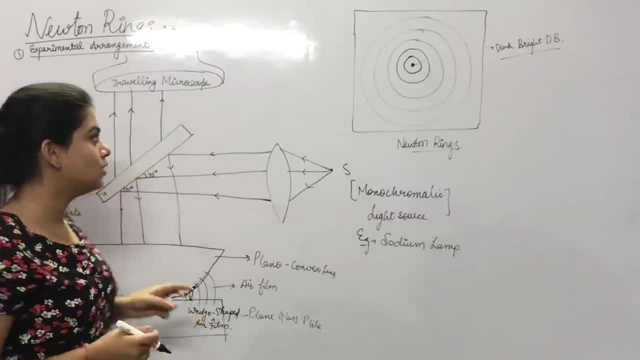 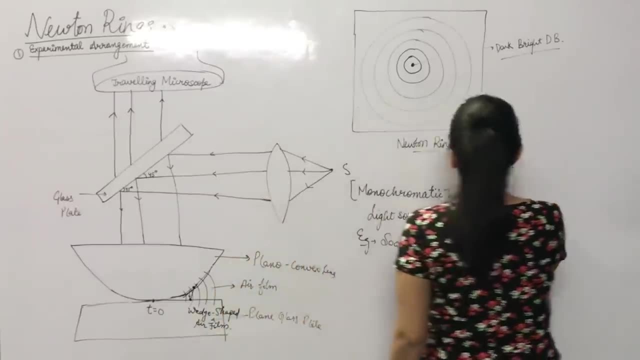 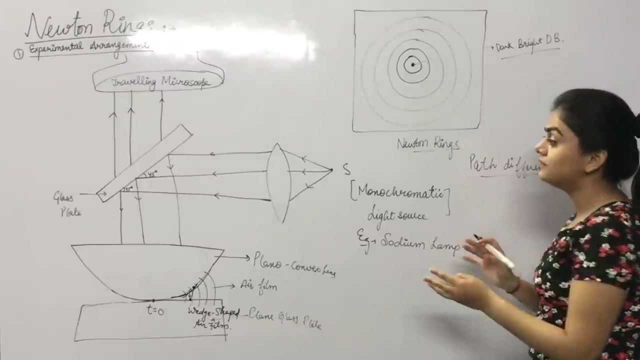 So now we are studying this in a reflected system, So let us calculate its path difference. To calculate the path difference, we know what is the formula of path difference in a reflected system: Path difference, What is the path difference? So it will be like this: 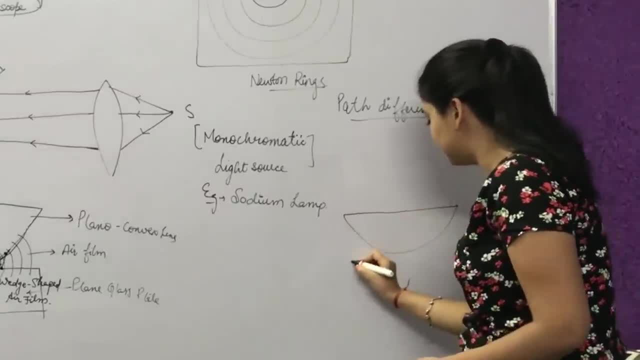 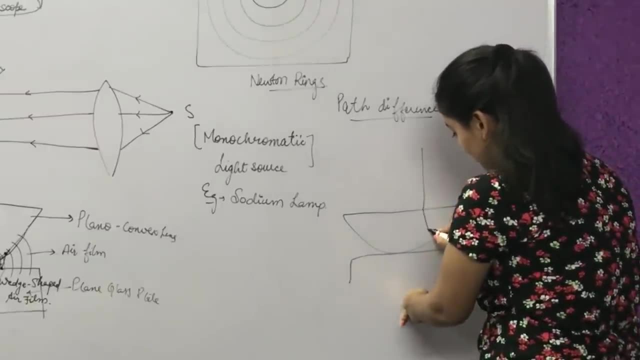 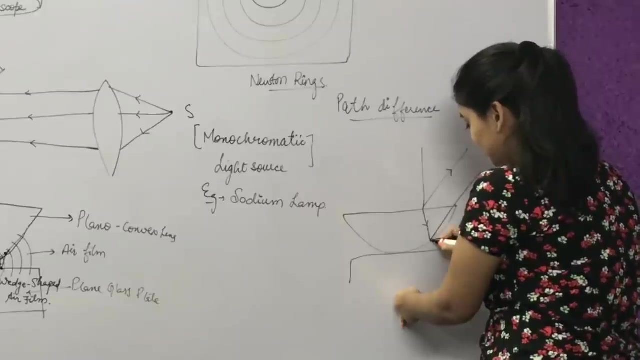 So if I have a ray, then this will be the path. So I will give you an example of a path difference of this kind. So if we have a ray now and I have an arrangement here, So I have a ray. 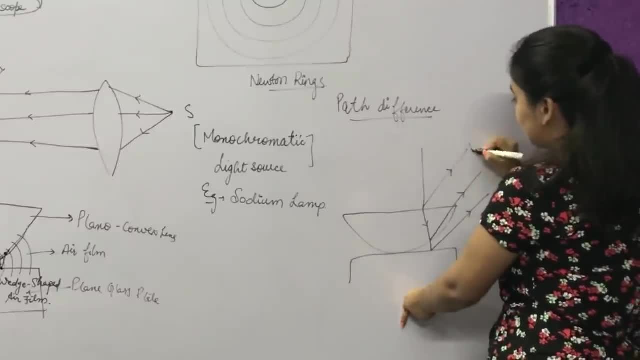 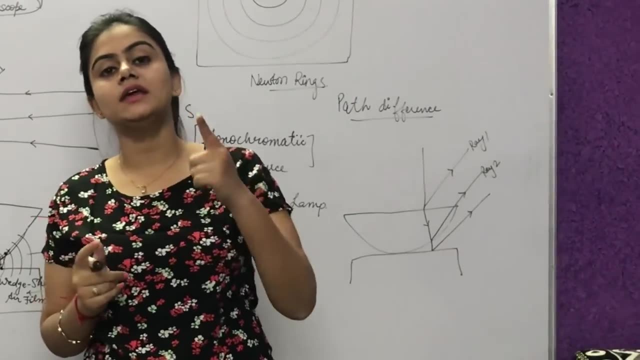 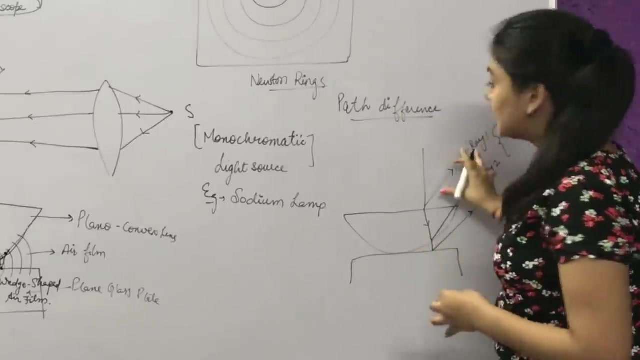 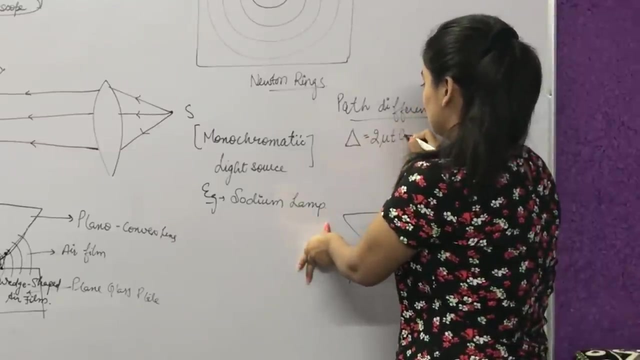 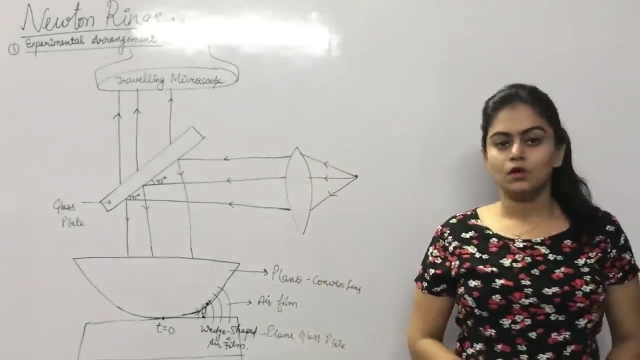 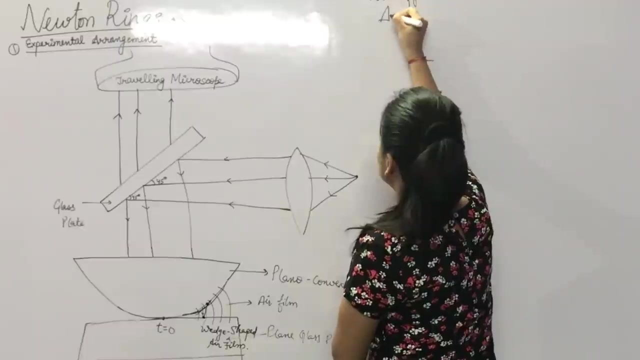 Partially it has reflected back and partially it has transmitted. So we will calculate the path difference between these two rays by the formula. delta is equal to 2 mu, t, cos r. So for reflected system we have the formula of path difference. delta is equal to 2 mu. 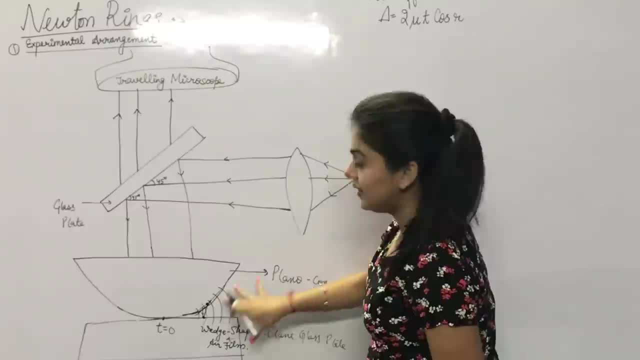 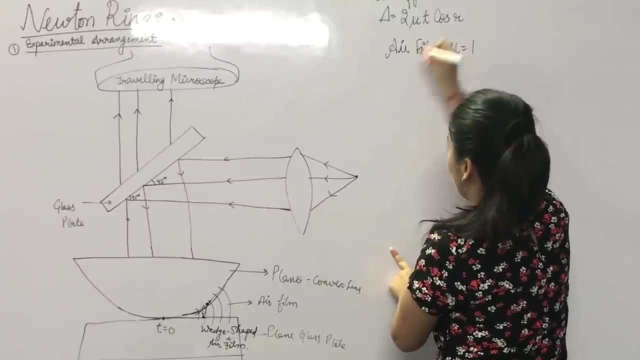 t cos r. So because here air film is forming, for air film mu is equal to 1 and we have the condition of normal incidence. So for reflected system we have the formula of path difference. delta is equal to 2 mu. 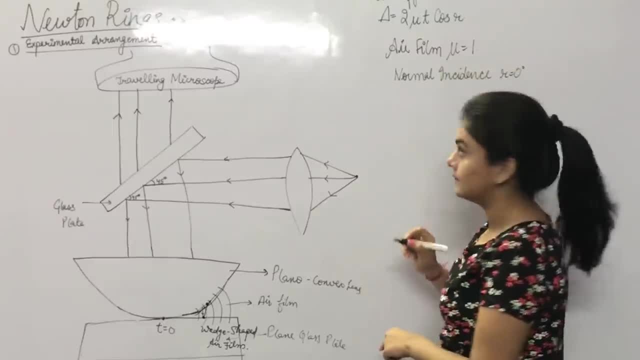 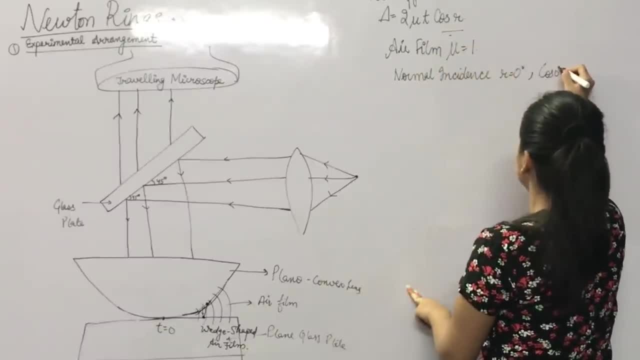 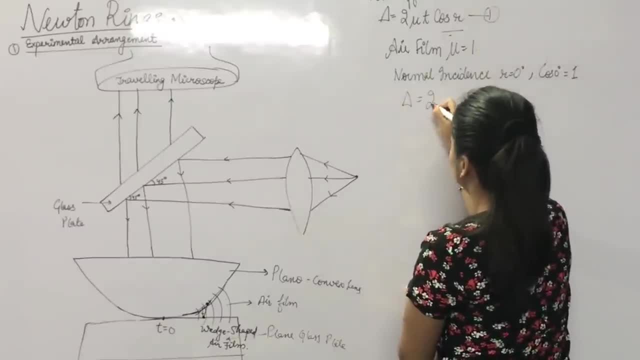 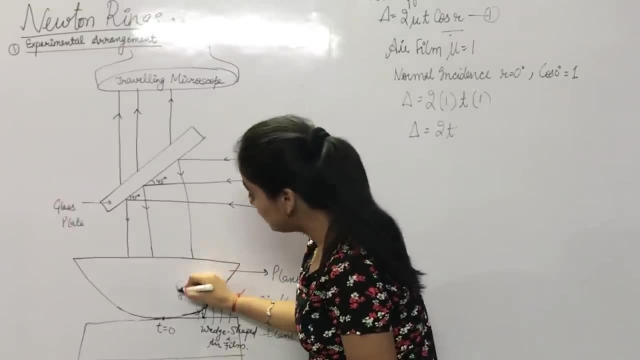 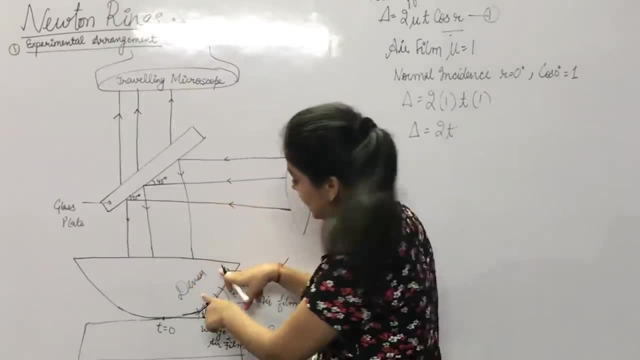 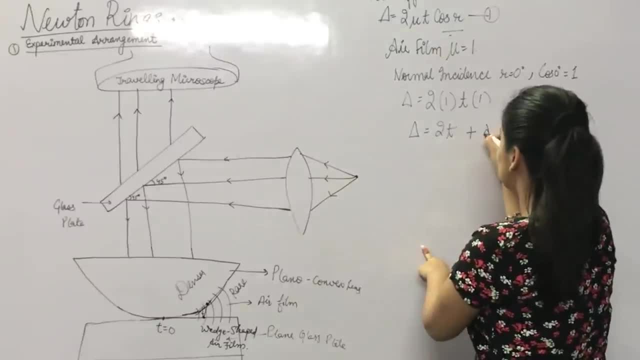 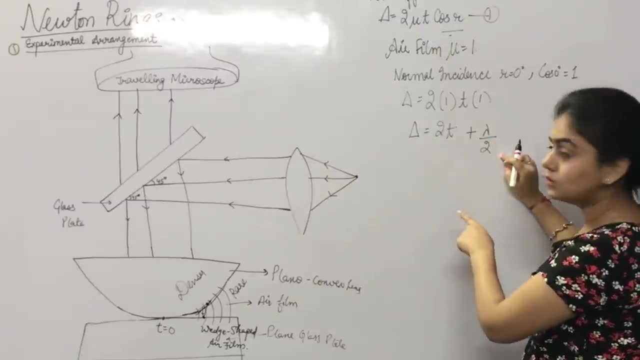 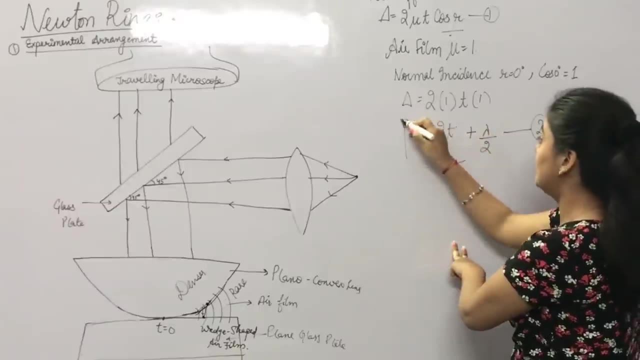 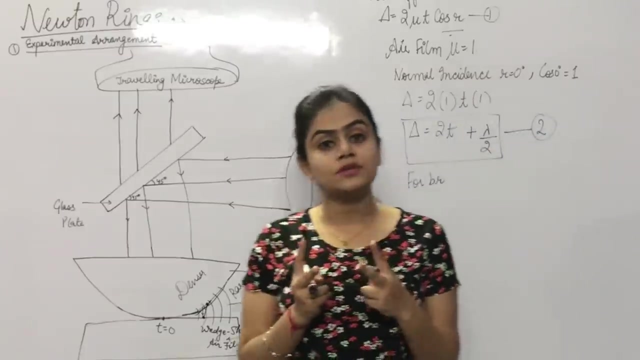 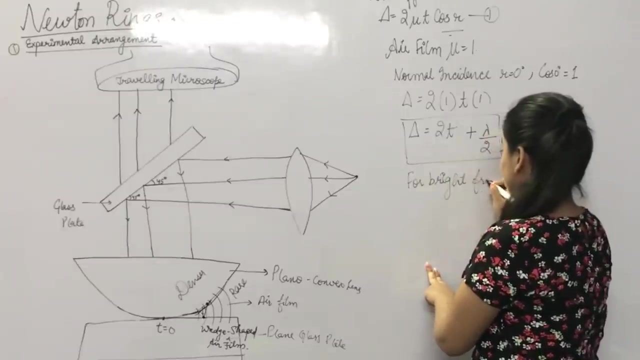 Therefore we have to write additional path difference that is denoted by lambda, by 1 trap aircraft term. So we have final path differenceケequation hvad delta is equal to 2t plus lambda by 2.. So for bright fringes, 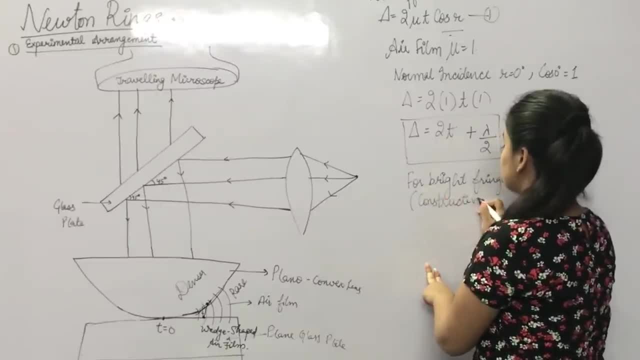 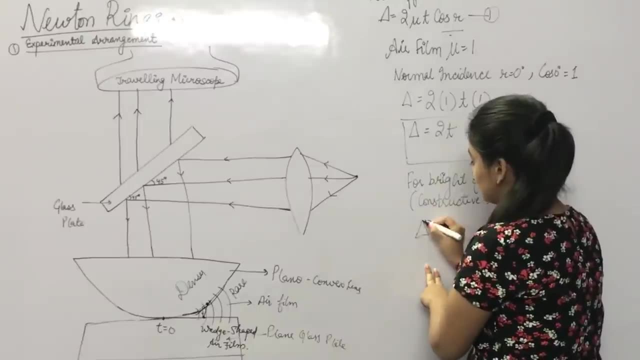 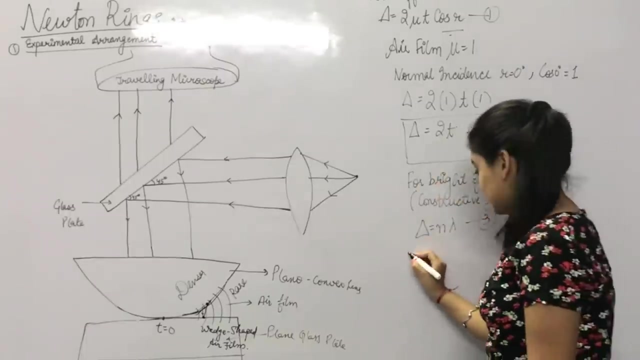 interference, Constructive interference, The two rays which we are talking about. there will be constructive interference between them. So the condition of constructive interference is delta is equal to n lambda Right. So equating equation number 2 and equation number, 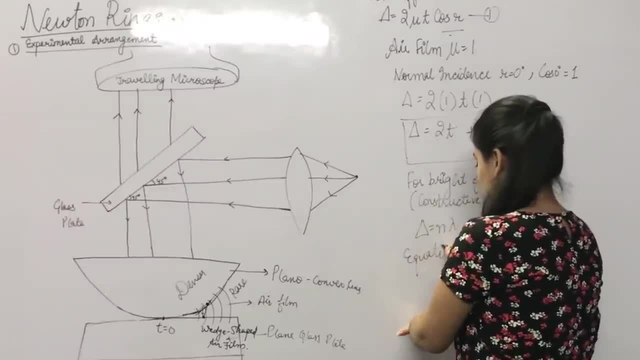 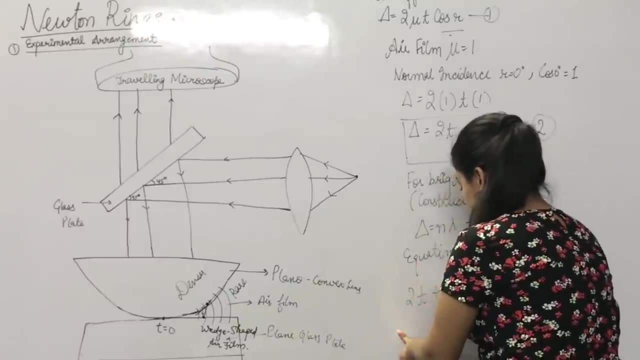 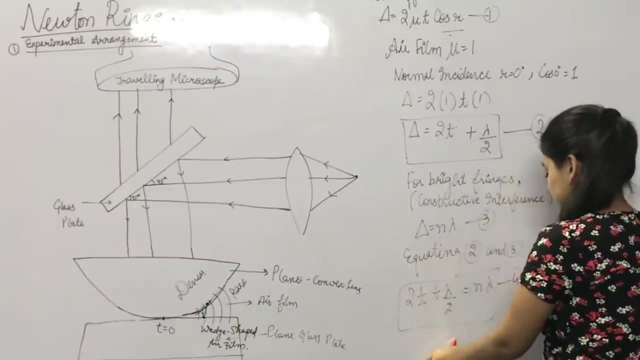 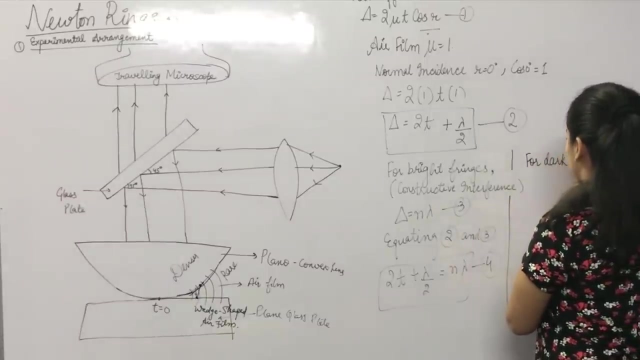 3, equating 2 and 3, we get 2t plus lambda by 2 is equal to n lambda. Equation number 4.. Right, So similarly for dark fringes, how do we have to do interference Constructive? 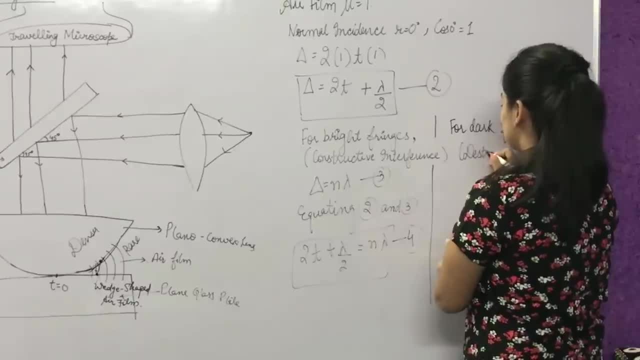 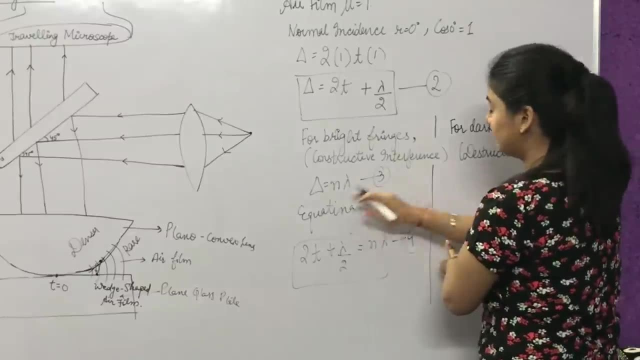 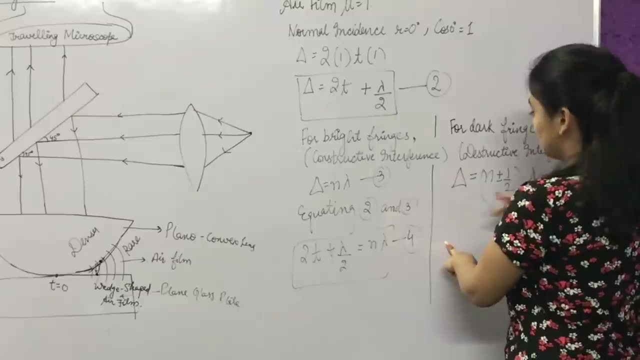 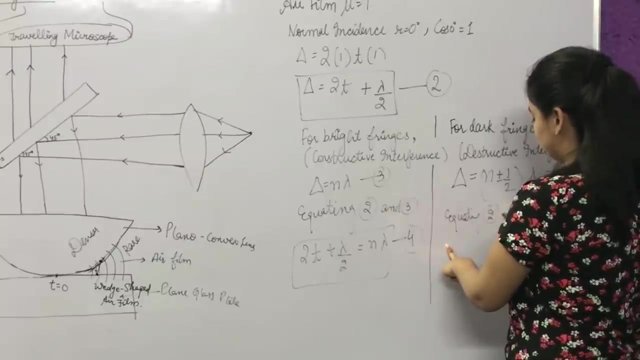 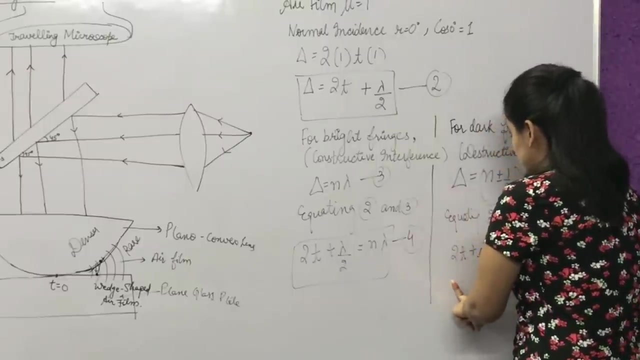 interference, Constructive interference. What is the condition of constructive interference? Constructive interference has the condition that path difference must be equal to n plus minus half lambda. So equating equation number 2 and 5.. Equating 2 and 5. We get 2t plus lambda by 2 is equal. to n lambda Right. So similarly for dark fringes. how do we have to do? interference? Constructive interference. What is the condition of constructive interference? Constructive interference. What is the condition of constructive interference? Constructive interference, Constructive interference. What is the condition of constructive interference? Constructive interference. 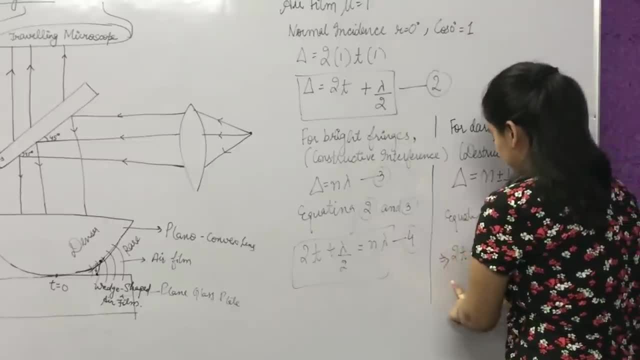 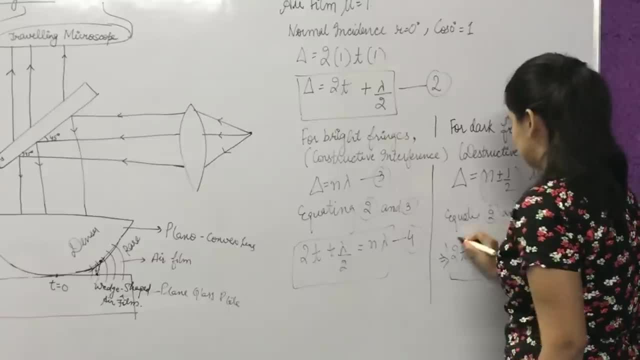 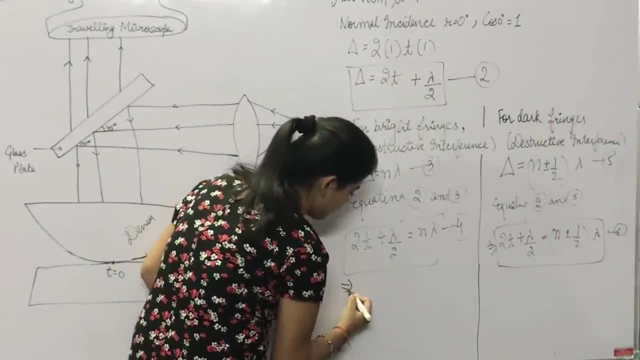 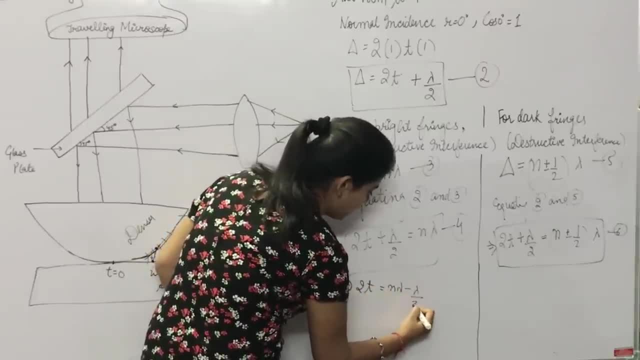 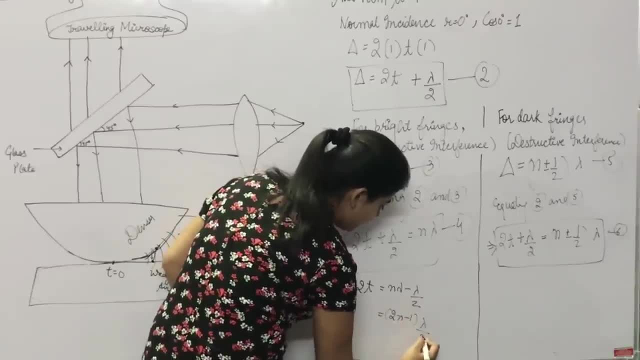 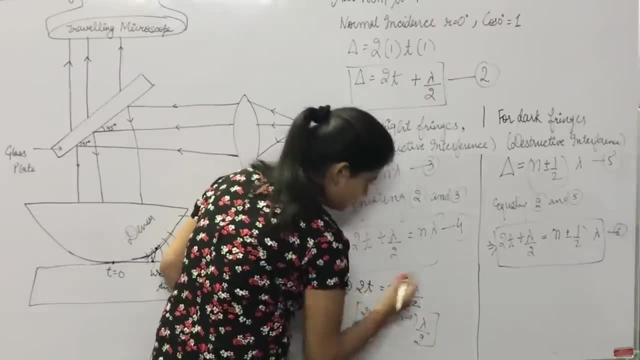 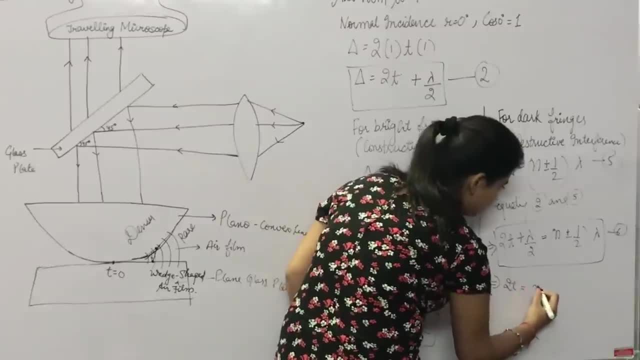 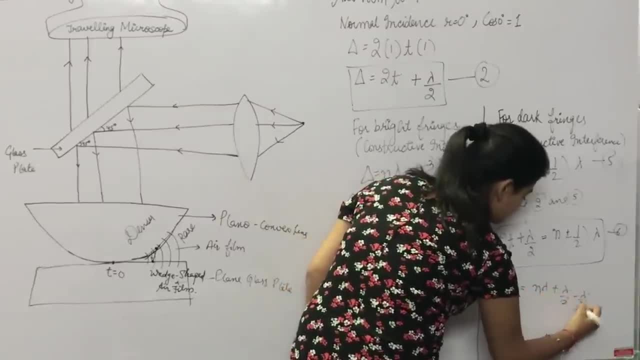 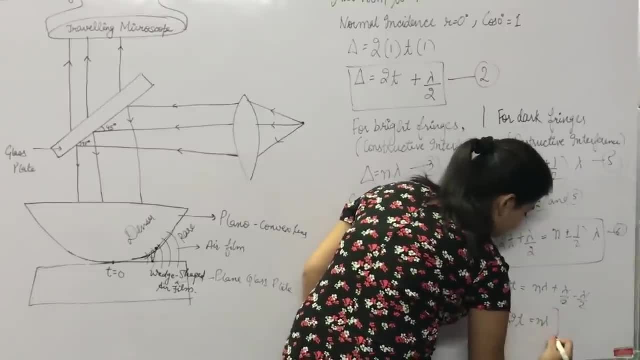 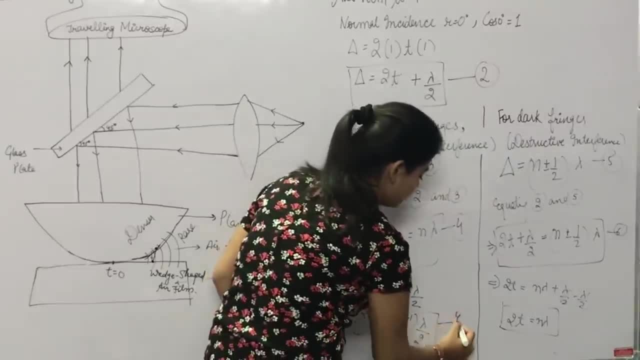 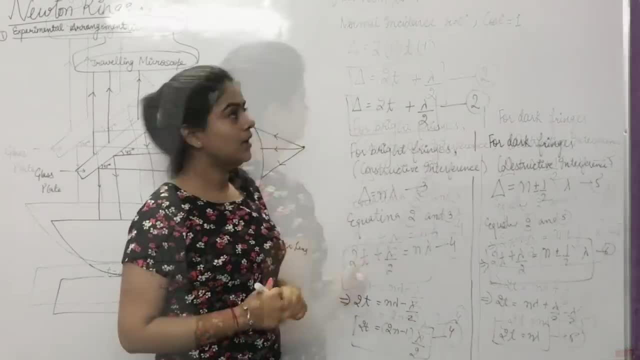 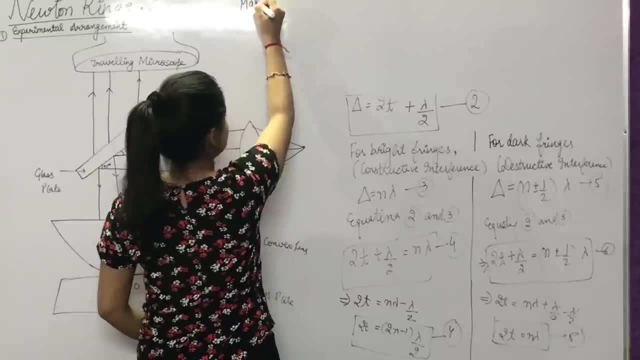 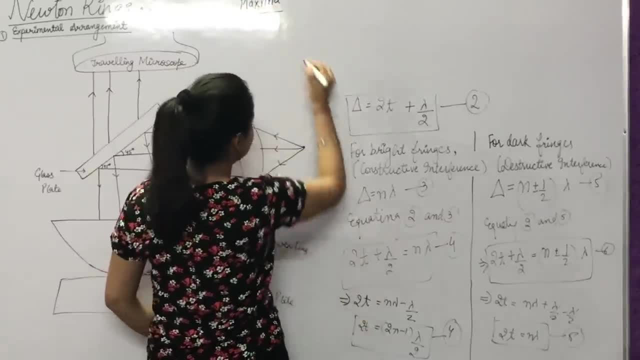 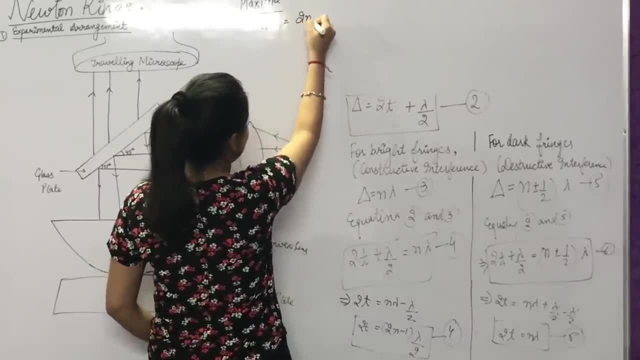 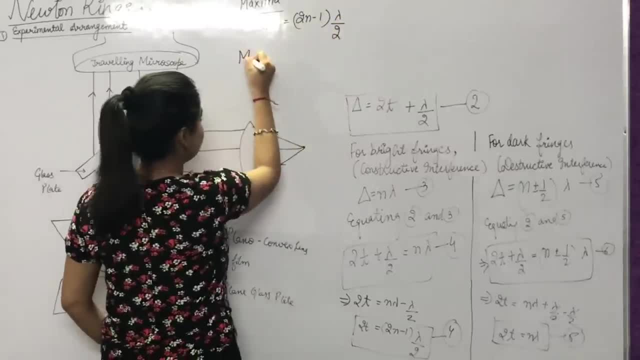 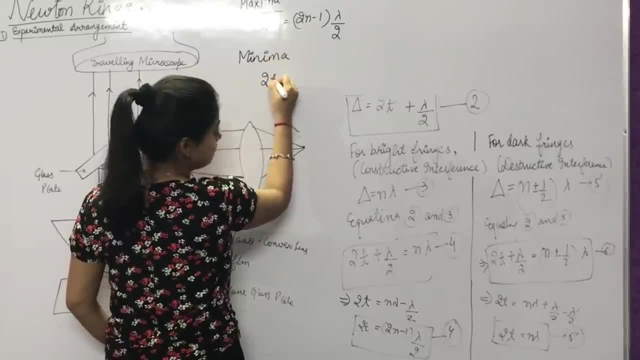 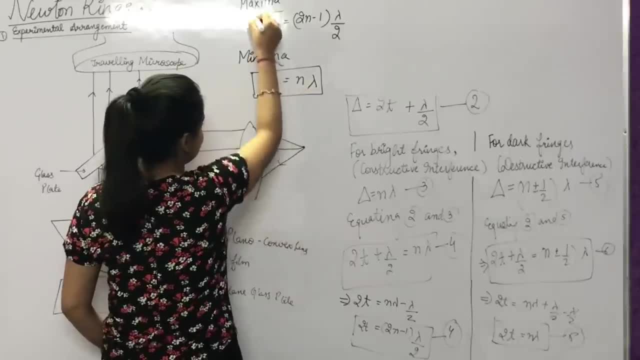 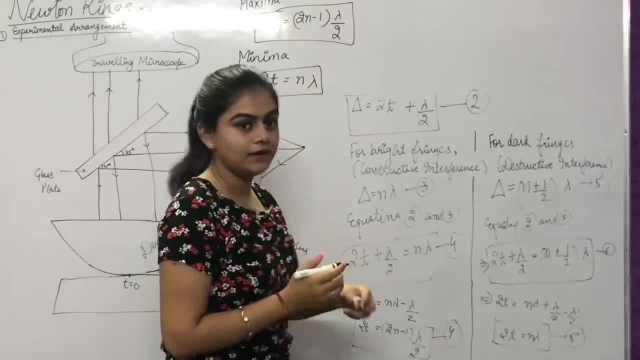 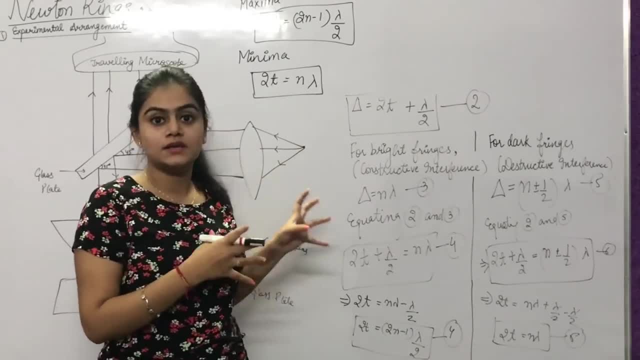 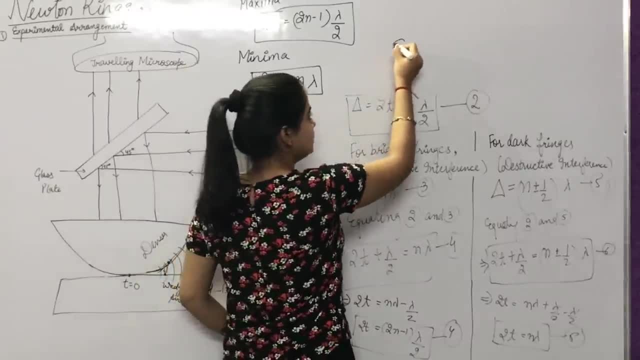 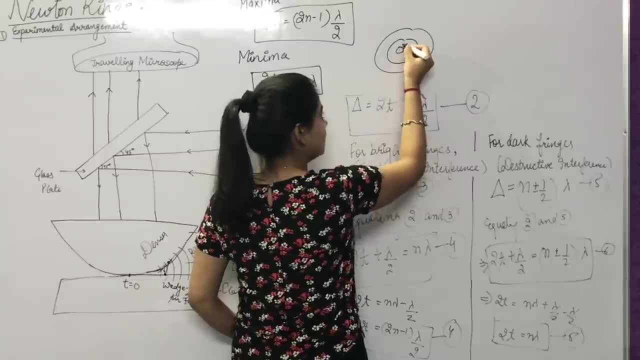 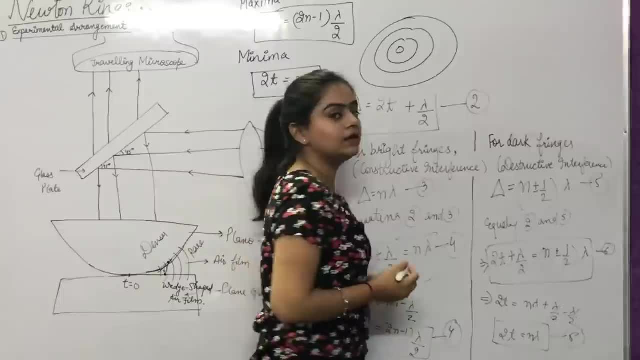 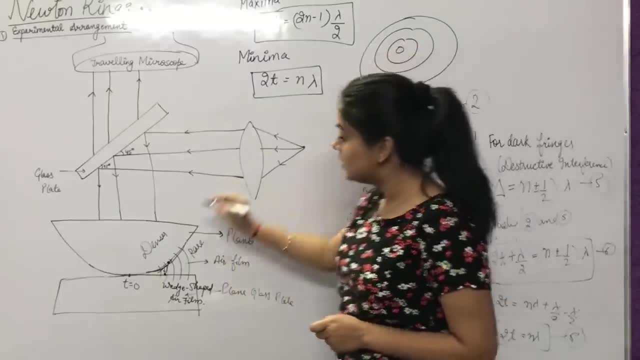 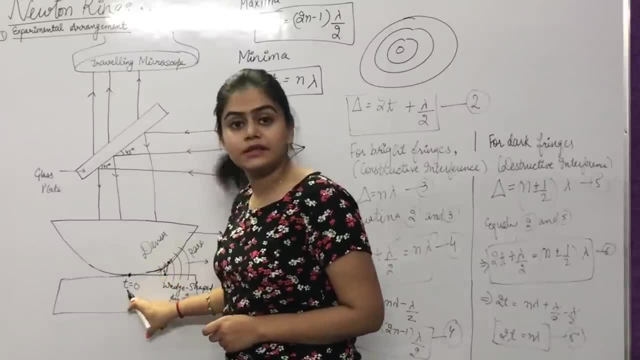 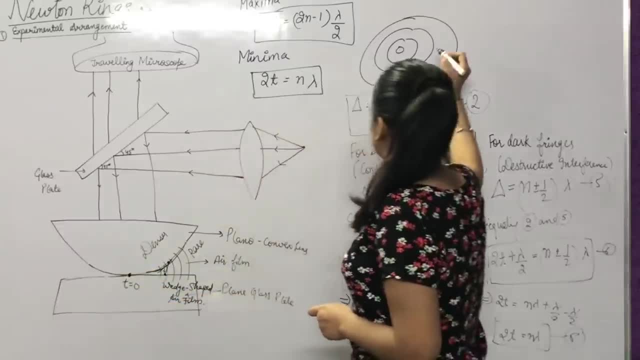 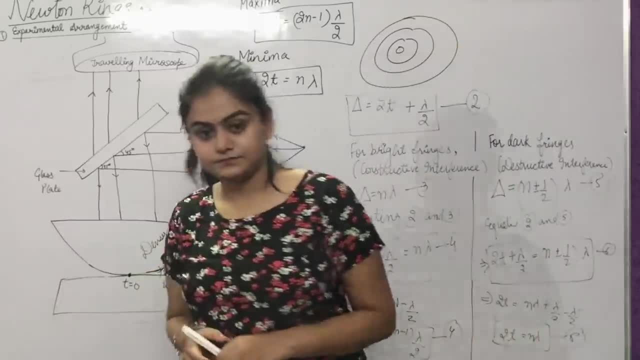 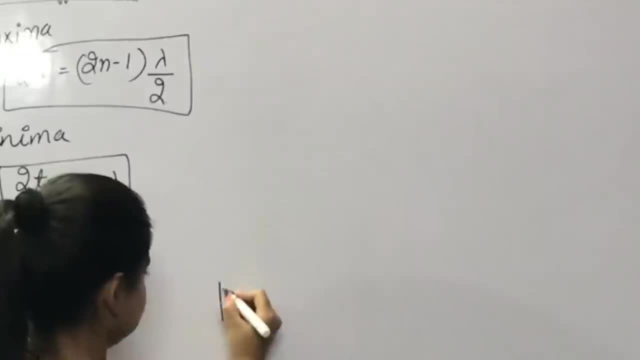 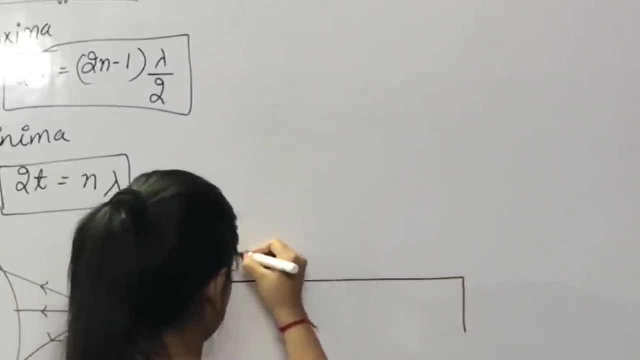 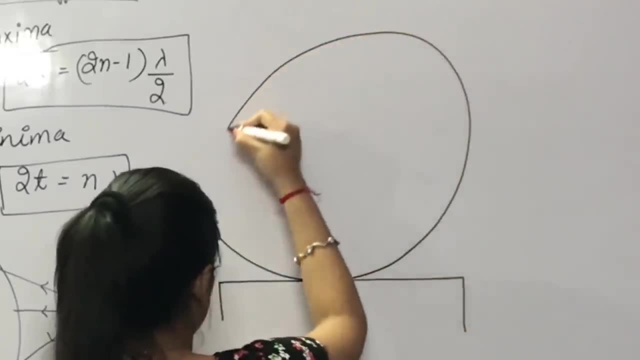 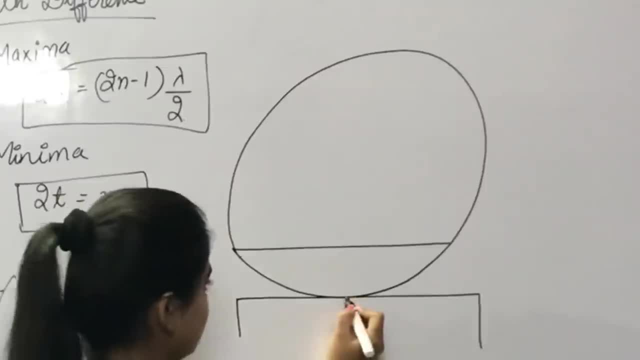 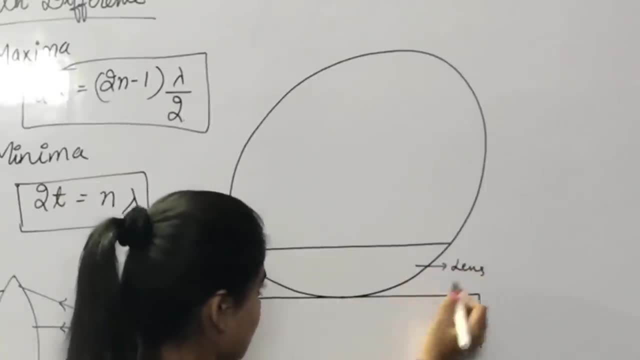 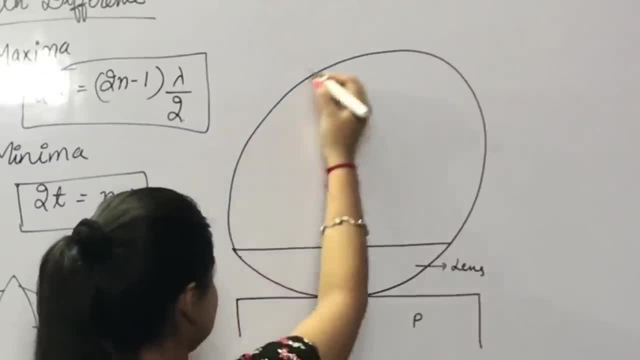 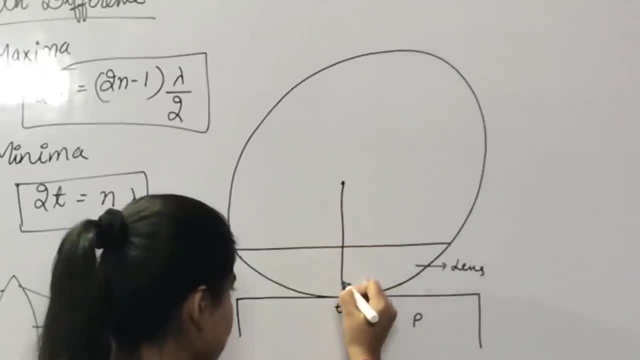 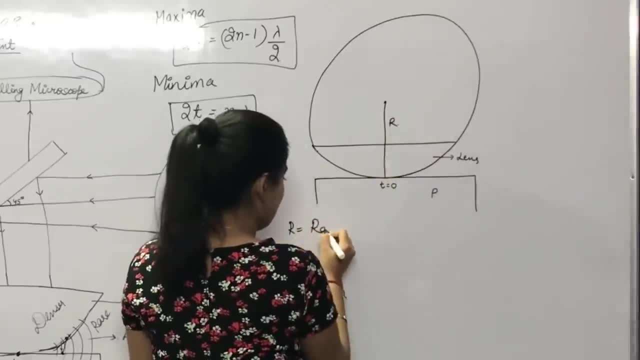 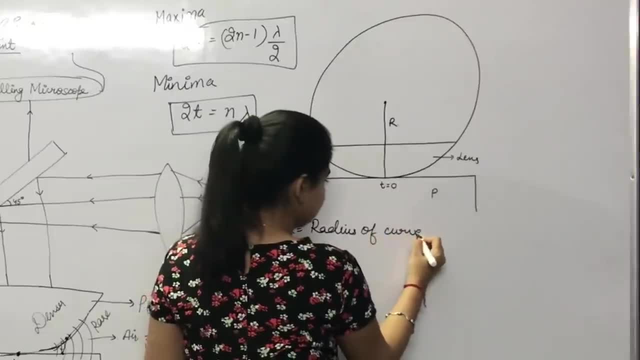 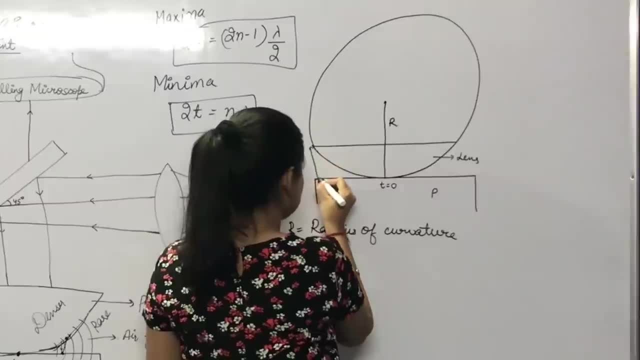 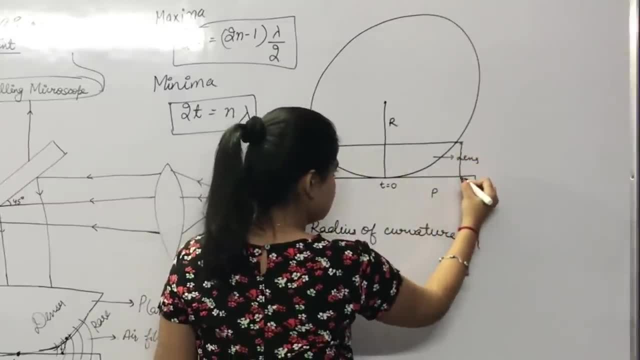 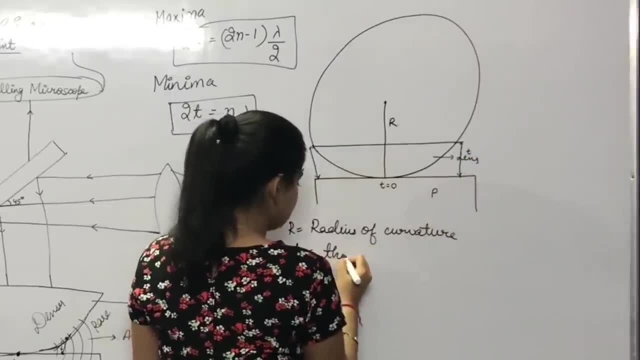 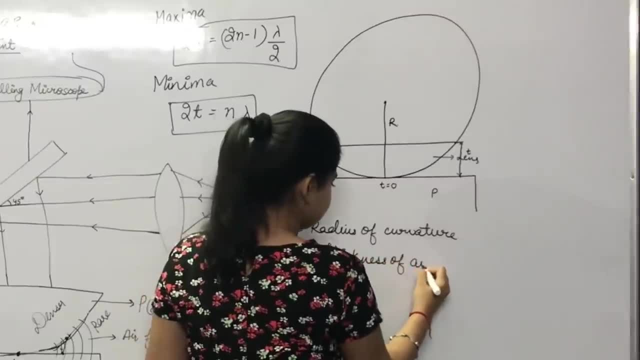 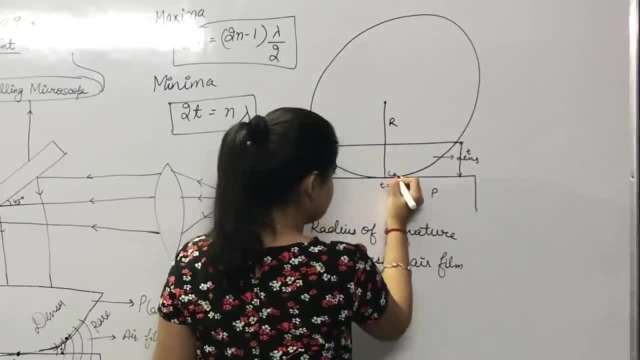 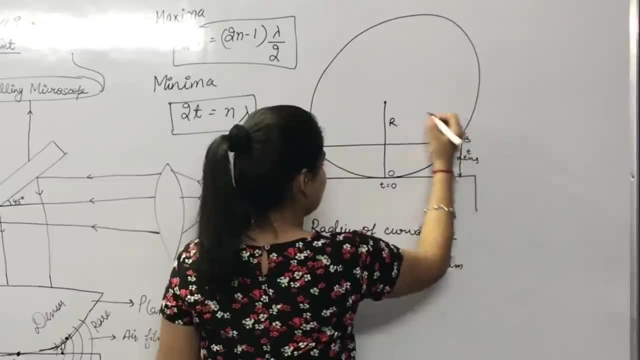 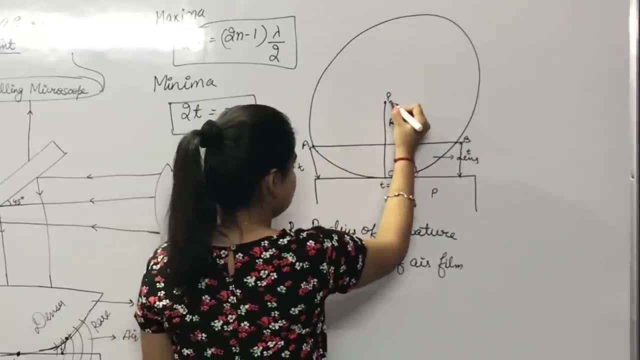 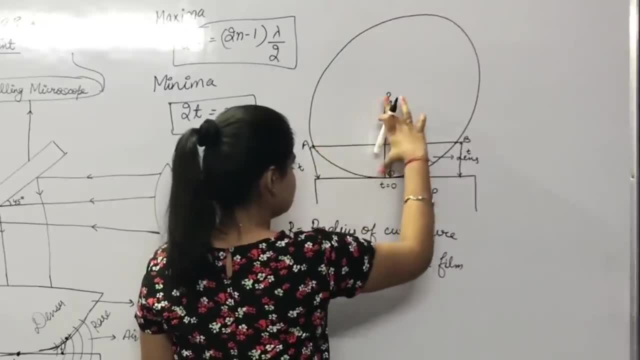 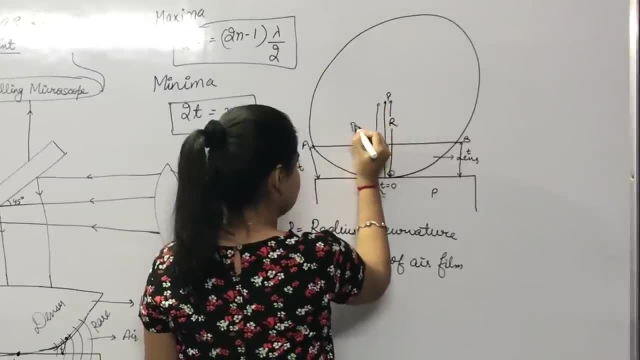 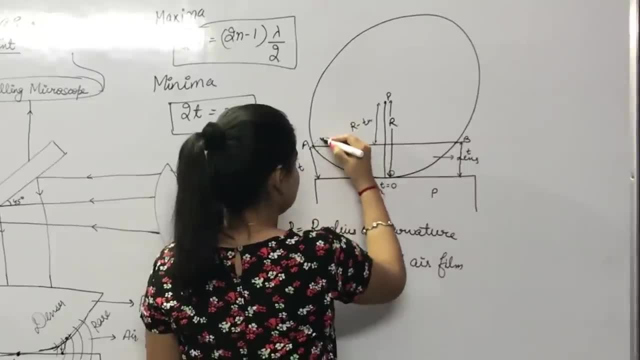 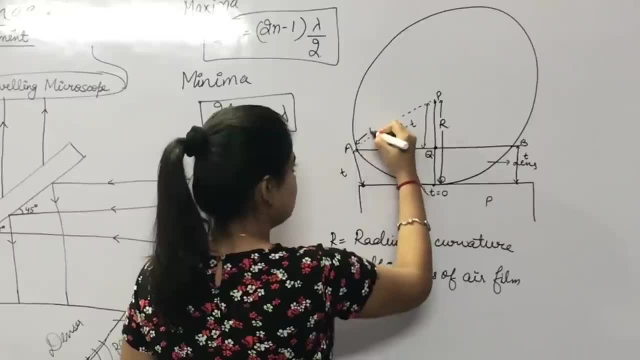 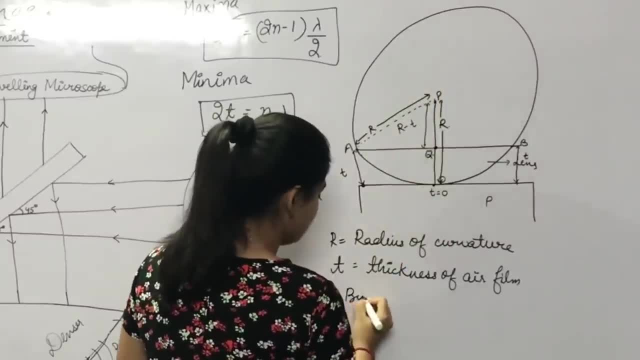 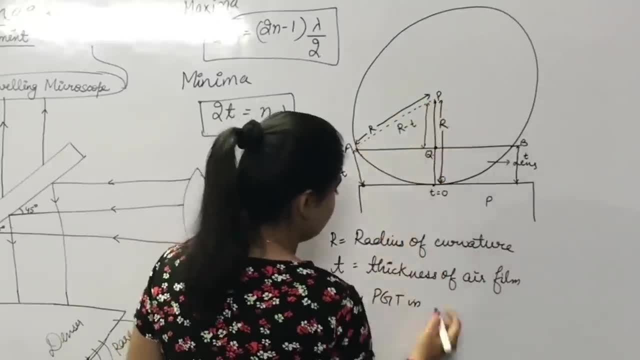 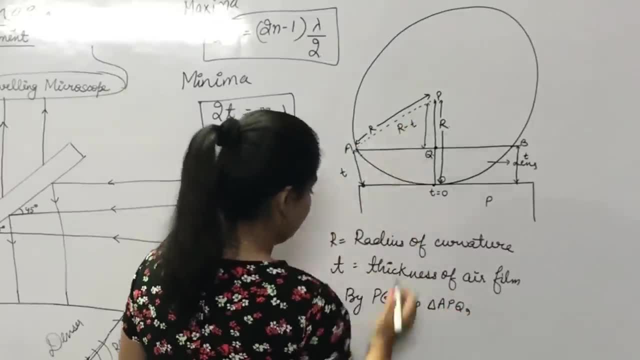 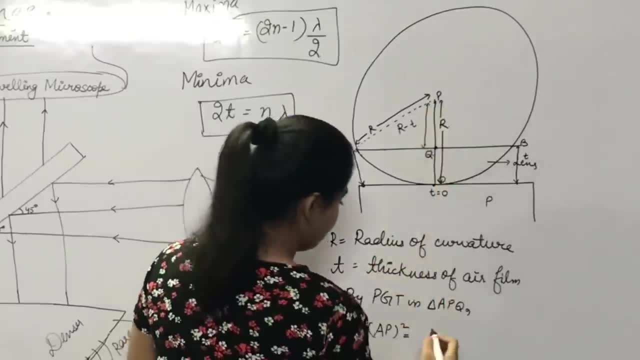 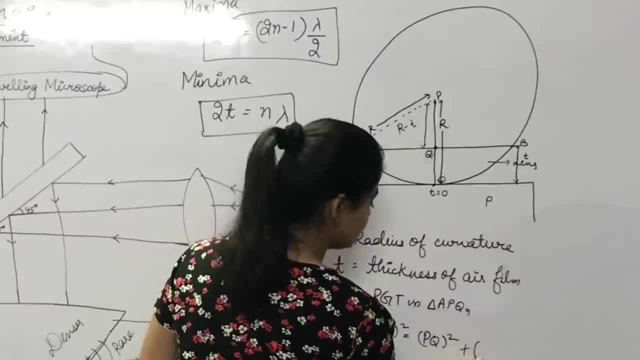 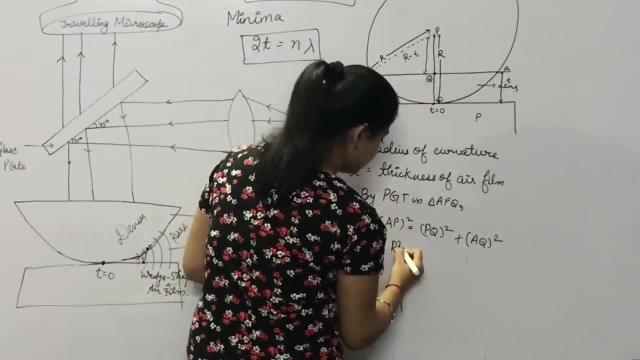 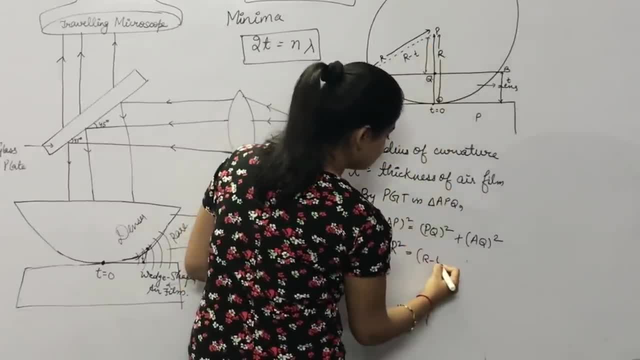 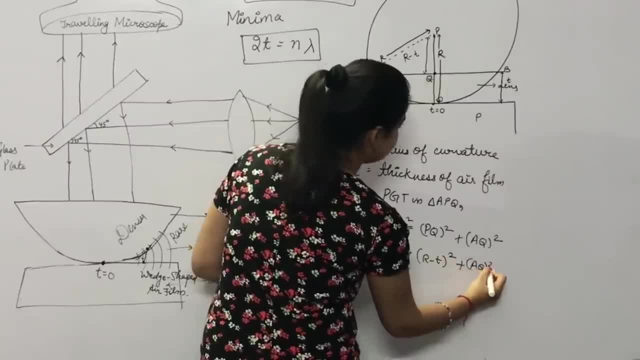 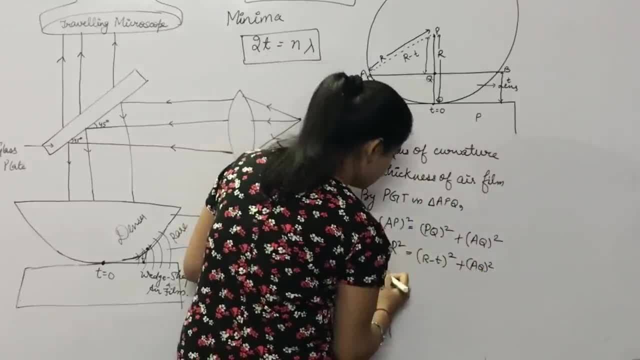 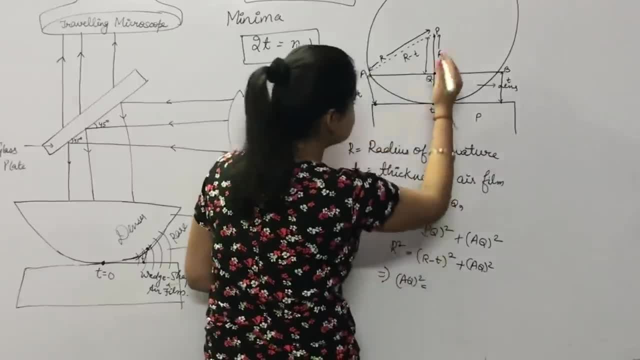 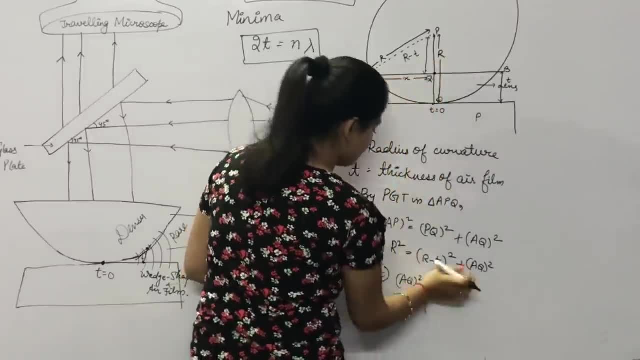 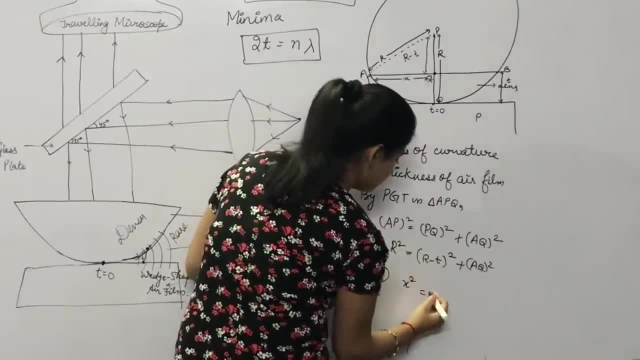 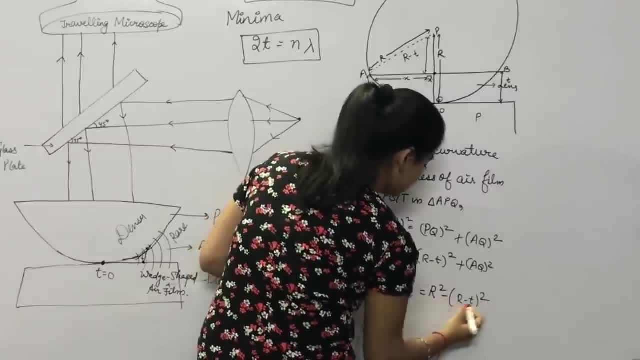 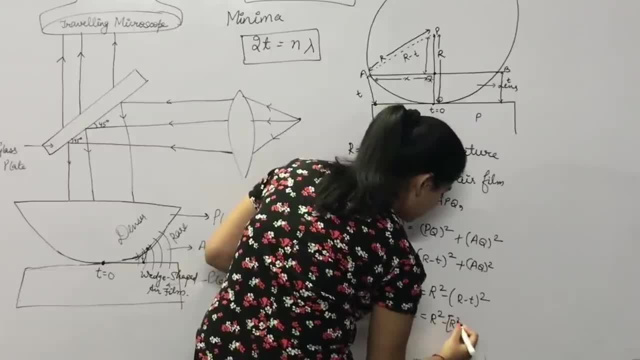 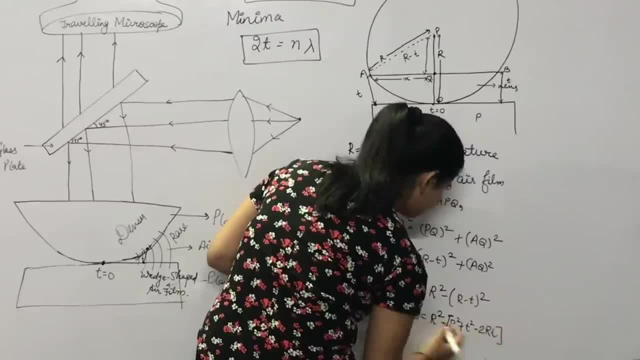 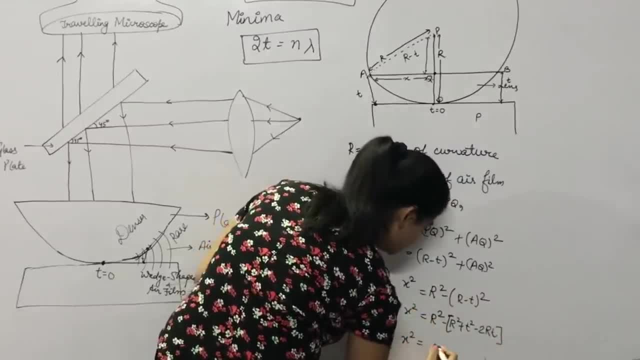 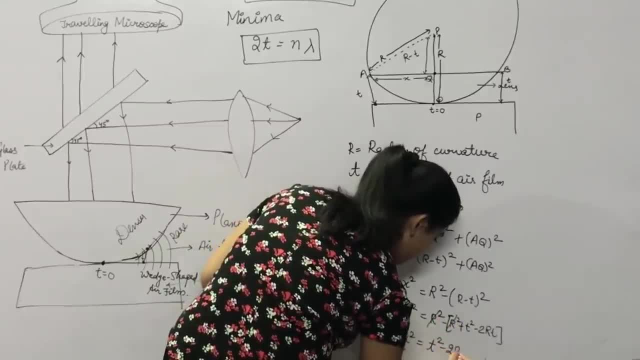 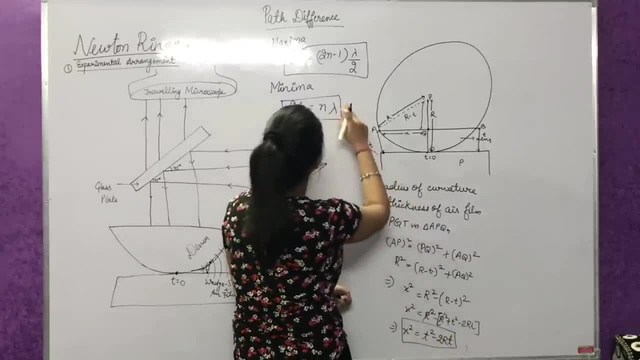 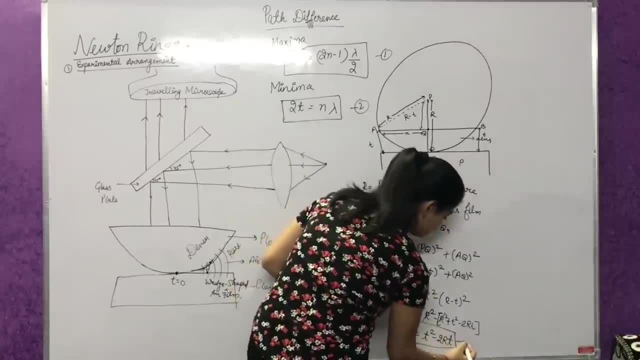 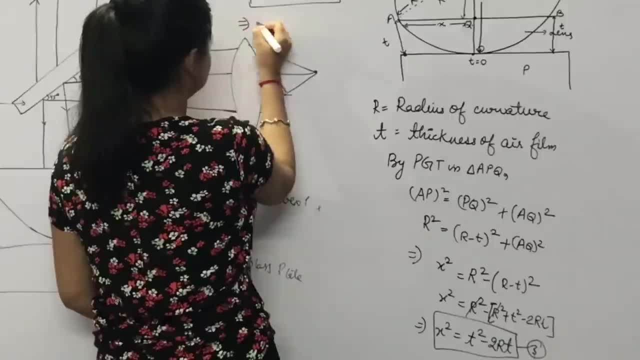 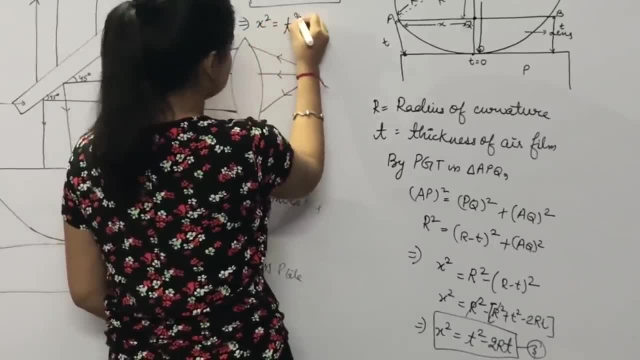 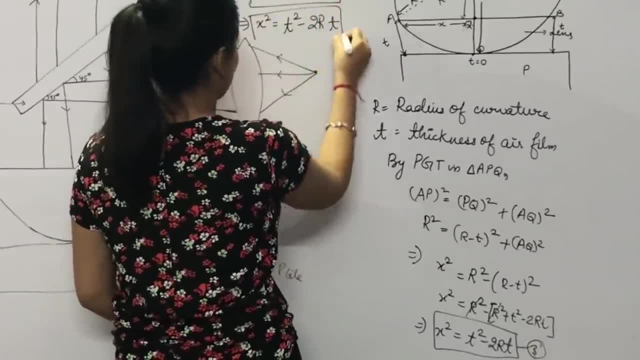 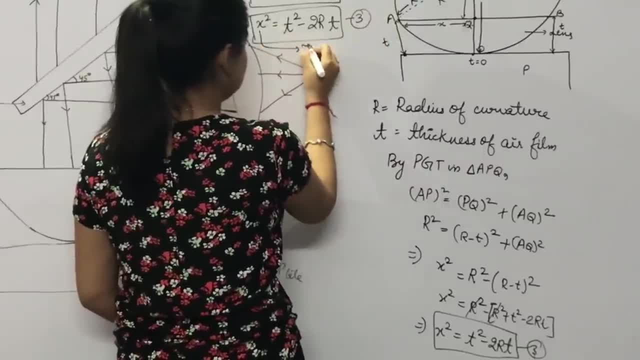 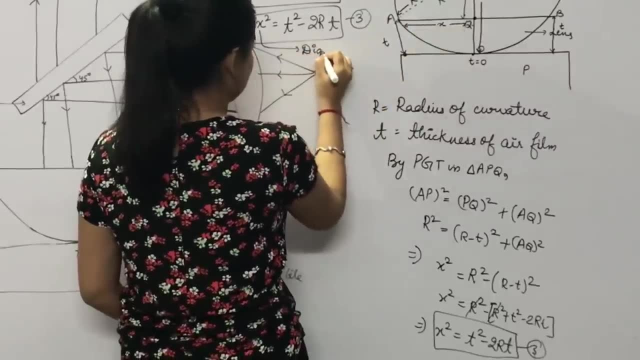 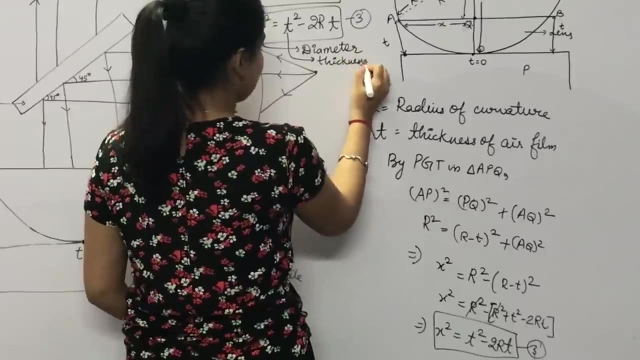 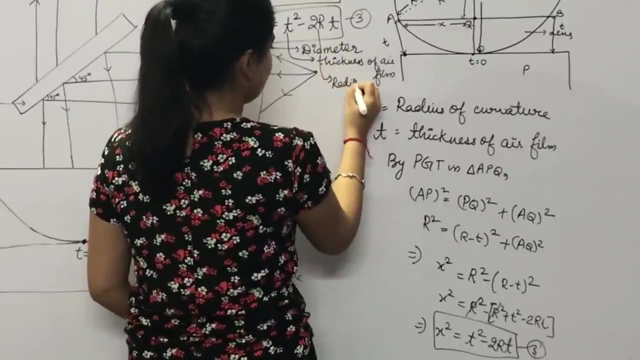 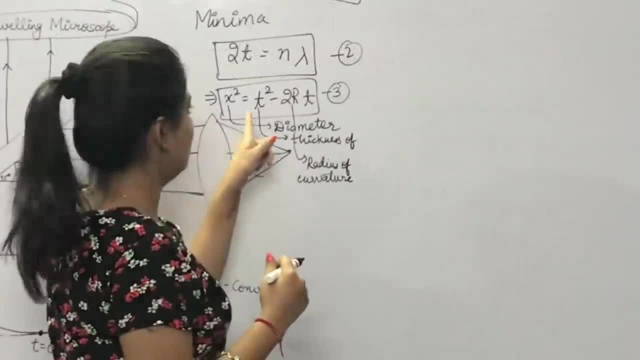 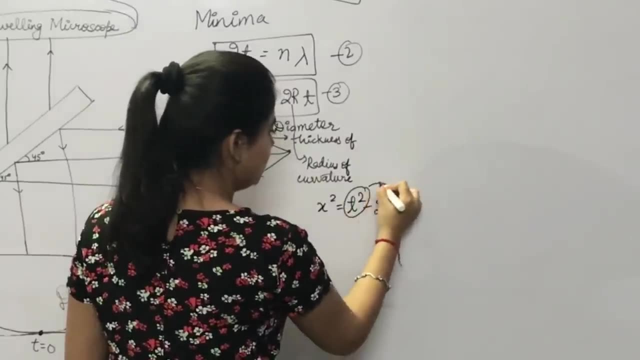 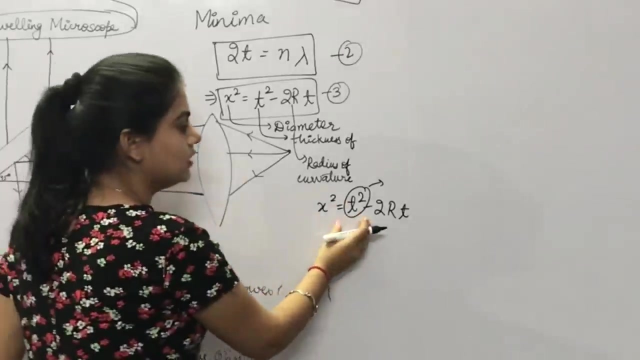 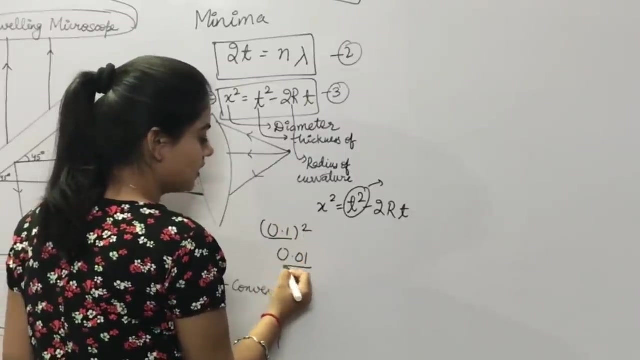 move on. So we have got x square is equals to t square minus 2 RT, Since t is what t is: the thickness of air film. Air film already is so thick, So if we square it the value will be more. We have 0.1 value. When we square it, we get 0.01.. So this is smaller. 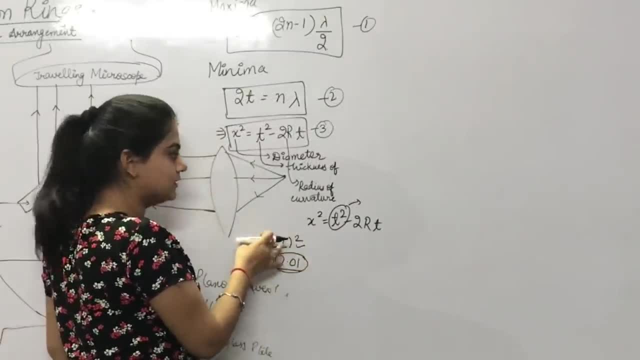 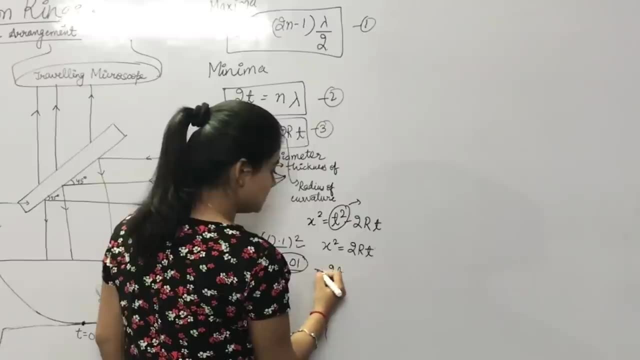 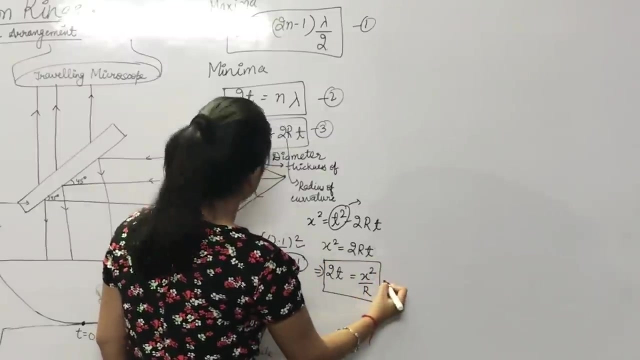 than this. The square of a small value is smaller than that, So we can neglect this term. So x square is equals to 2 RT. So from here, 2 t is equals to x square upon r, Equation number 4.. Now we can compare these two. So for maxima we can put x square upon 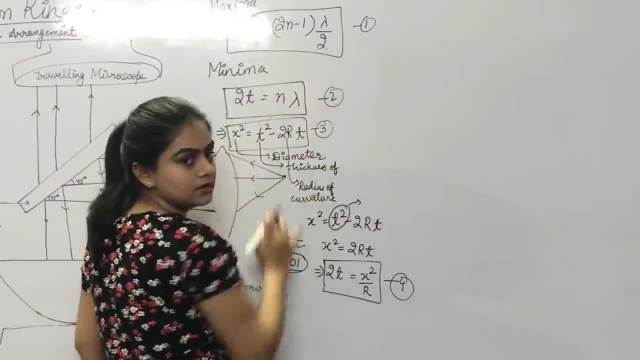 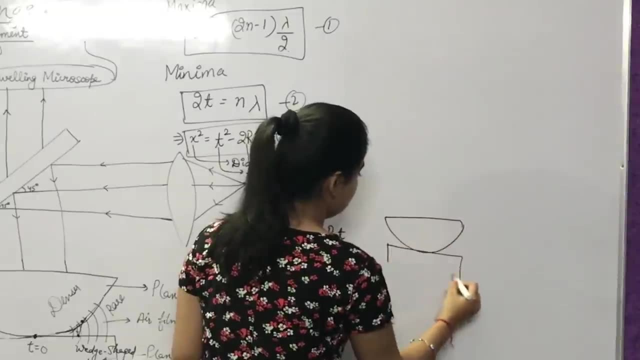 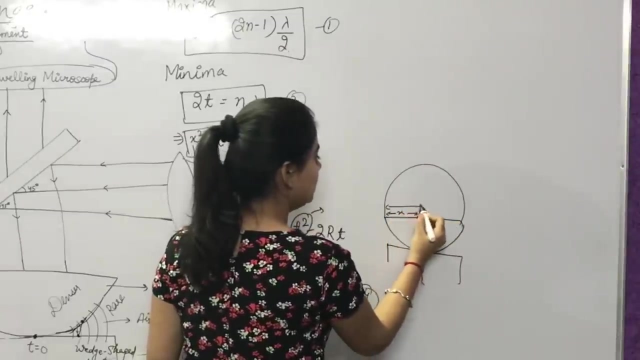 r is equals to this and for minima we can put it equal to this. So this is our x. The diagram which we had made, which was our x, that was this. This was x. So we have to talk about the complete diameter. So diameter d is equals to 2 x. 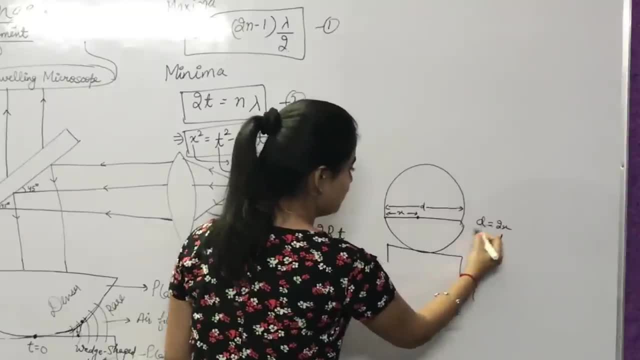 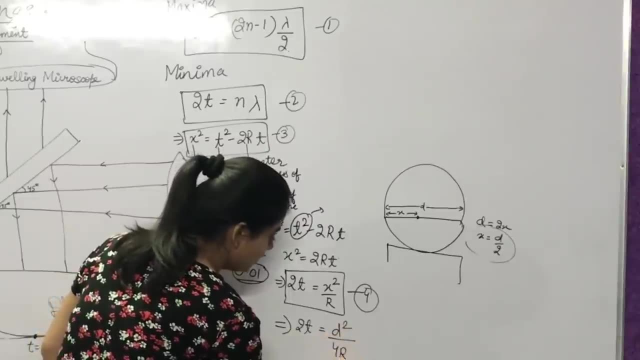 Can we write like this: And x is equals to d by 2.. So put x is equals to d by 2 in equation number 4.. So 2 t is equals to d square upon 4 r. Now for maxima, we can put x square. 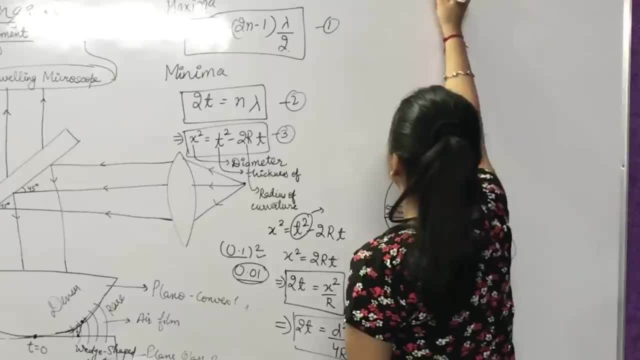 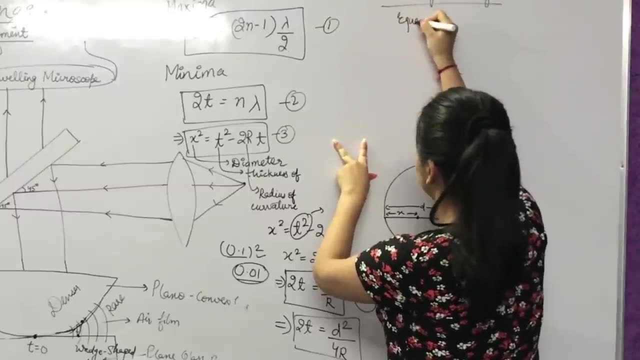 upon r. So 2 t is equals to 2 x. So 2 t is equals to 2 x. So 2 t is equals to 2 x For maxima for bright fringe, equating equation number 1 and equation number 4.. So we get. 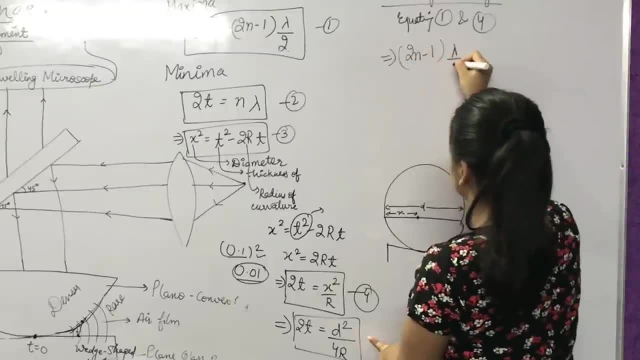 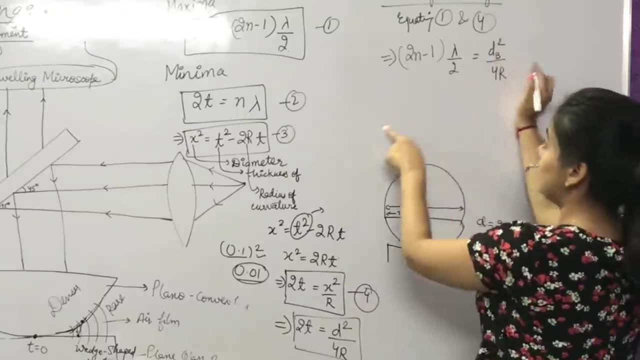 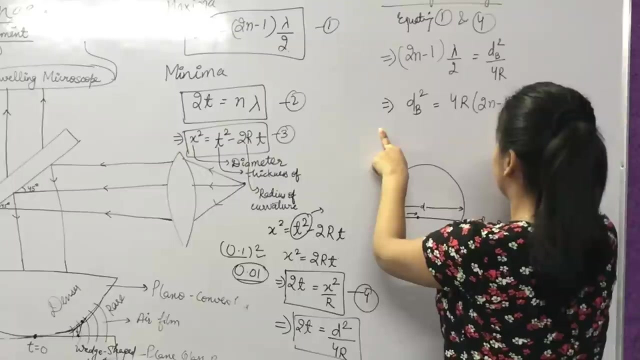 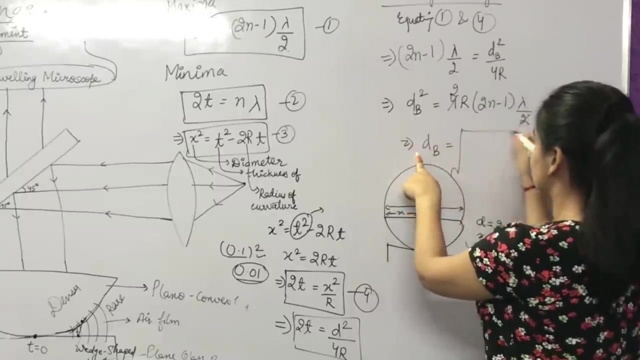 2 n minus 1 lambda by 2 is equals to d square upon 4 r. So this is for bright fringe. That's why I am writing b here. So d b square is equals to 4 r. 2 n minus 1 lambda by 2.. 2 cancels this. So d b is equals to: under root: 2 r, 2 n minus. 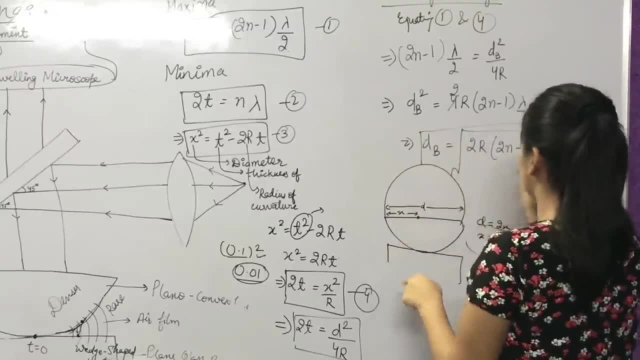 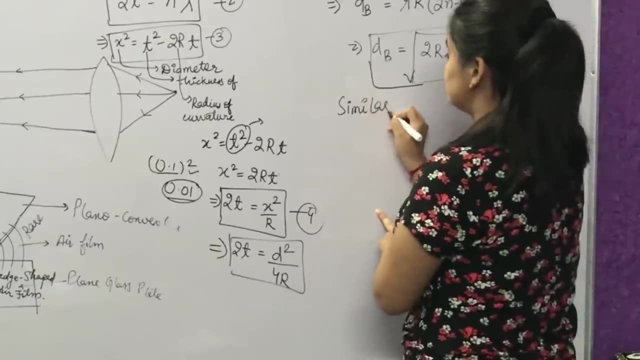 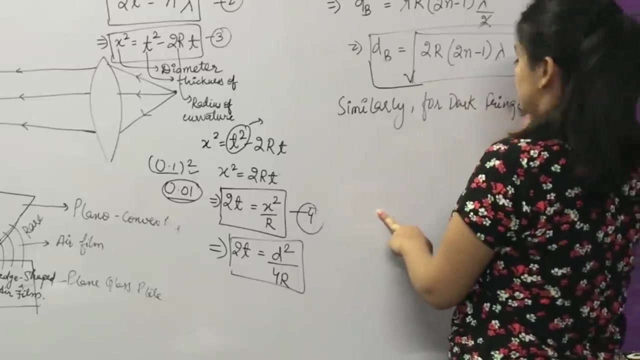 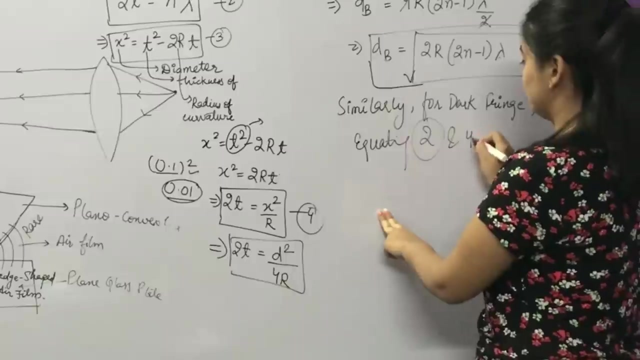 1 lambda. So this is the diameter for a bright fringe. Equation number 5.. So, similarly for dark fringe. For dark fringe, We will equate equation number 4 and equation number 2.. So equating equation 2 and 4.. So 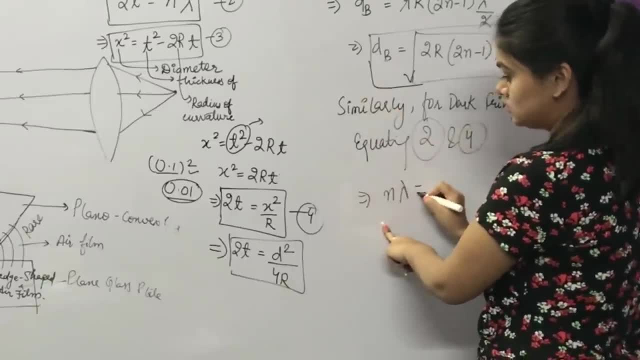 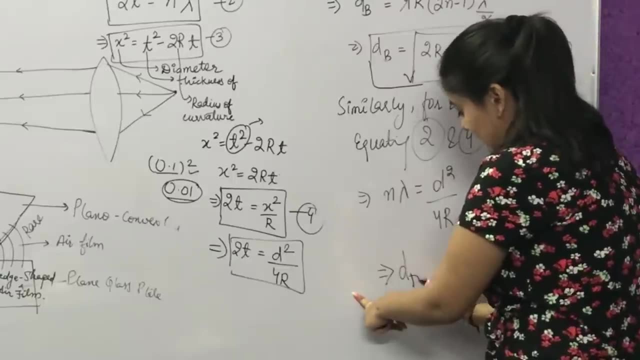 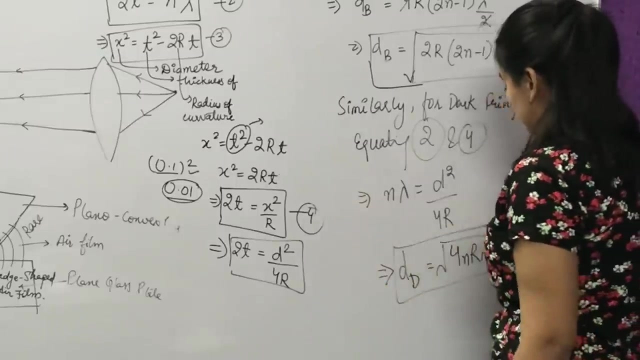 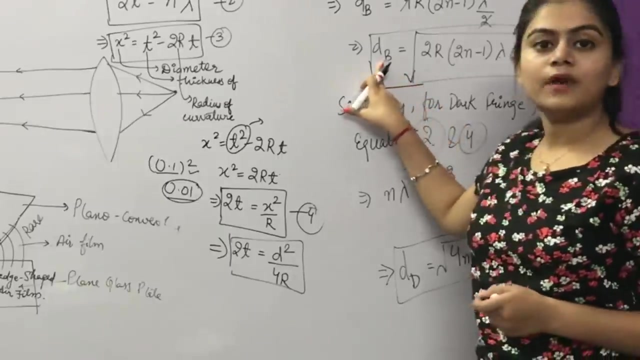 we will get n. lambda is equals to d square upon 4 r. So from here, d dark is equals to 4 n r lambda under the root. Let us give it equation number 6.. So we have got two formulas here. Diameter for bright fringe is given by the formula under: 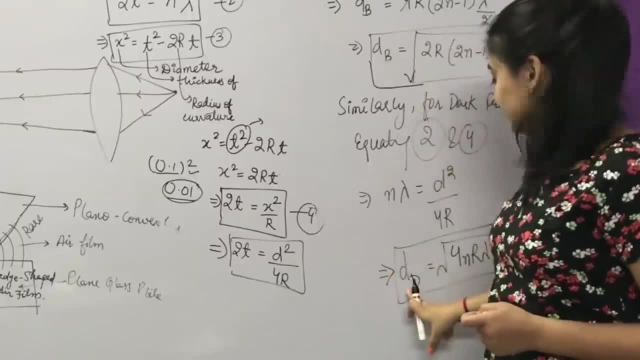 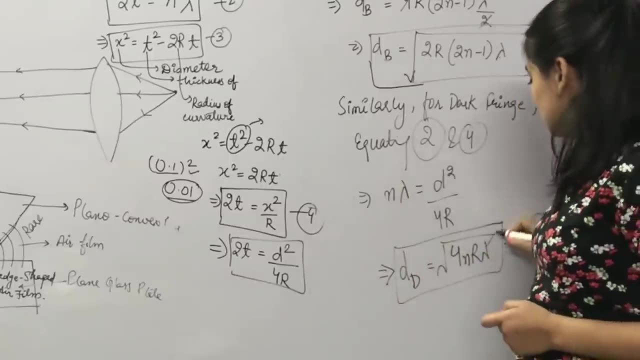 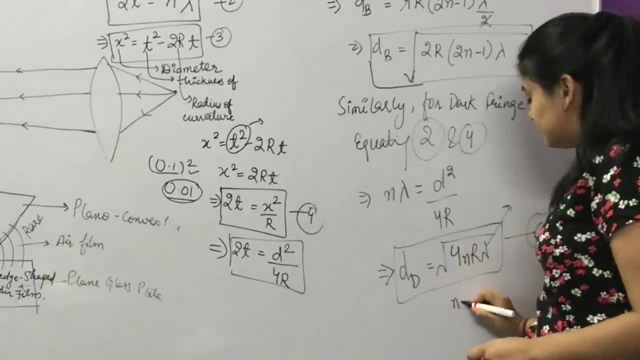 root 2 r, 2 n minus 1 lambda and diameter for dark fringe is given by under root 4 n r. lambda r is the radius of curvature of the lens and lambda is the wavelength of the light from the monochromatic light source. n can vary from 0,, 1,, 2,, 3 and so on. Right. 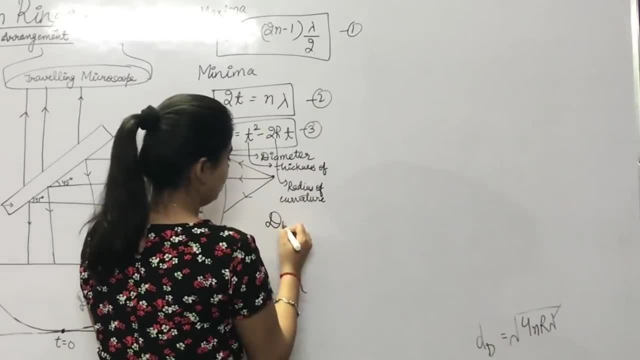 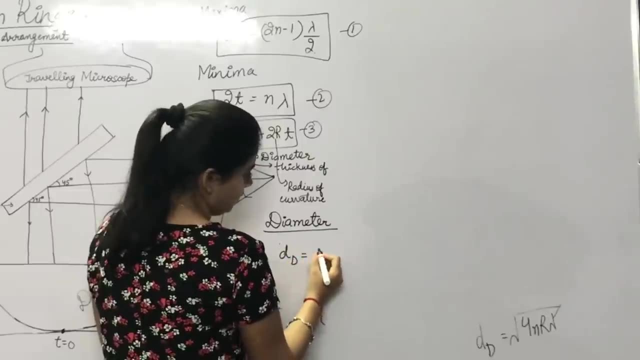 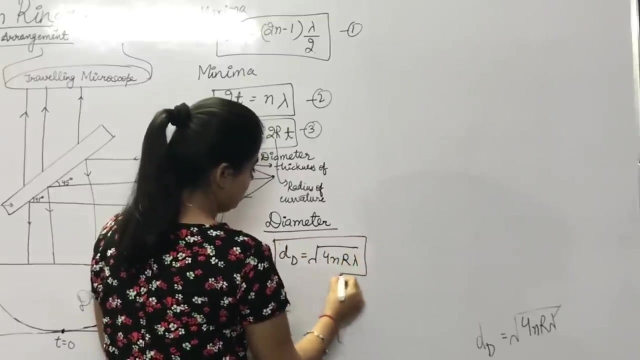 Right. So we have got one more formula here for determining the diameter. So for determining diameter we have got a formula for dark fringe: D is equal to 4nR lambda. So now we will find out how to determine the wavelength of the light used. 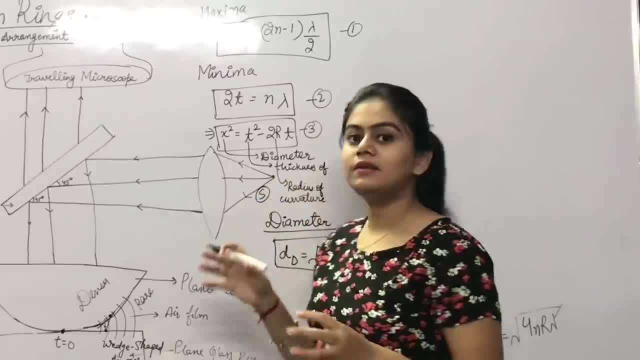 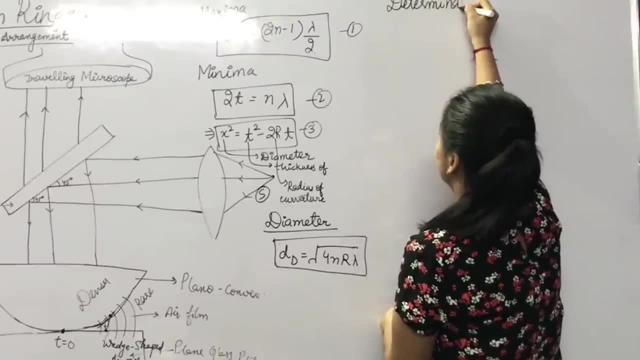 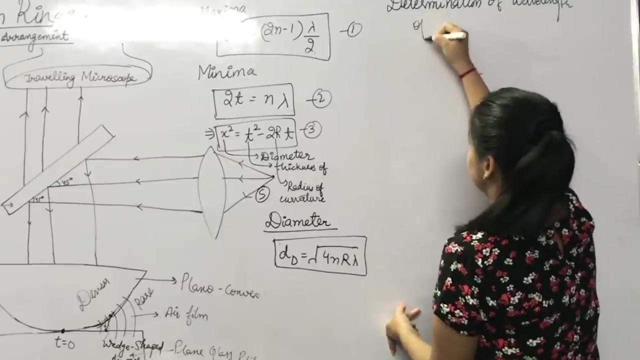 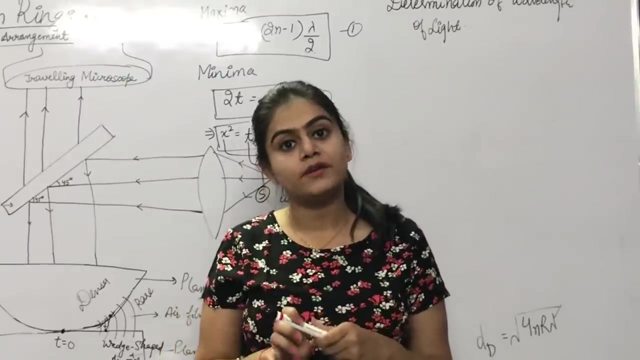 The light source which we have used. what is the wavelength of light coming from that light source? For that, what we will do is for determination of wavelength of light. we will take two consecutive dark fringes or two consecutive bright fringes. 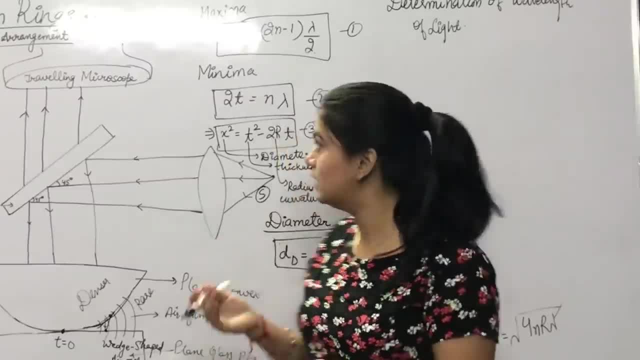 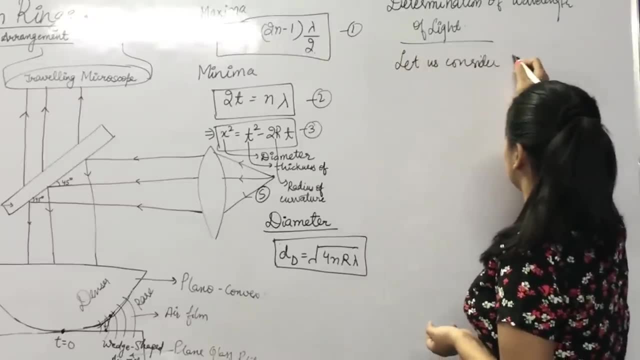 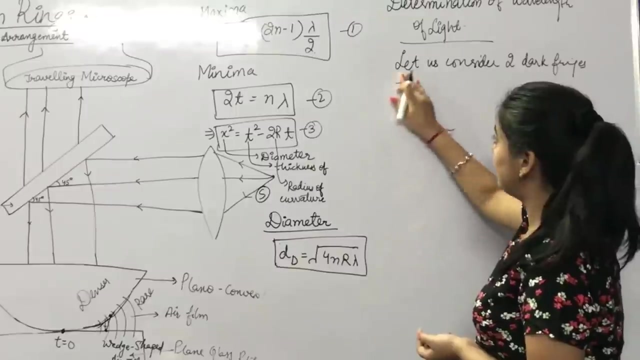 The distance between them will be the wavelength, So we will take two consecutive dark fringes. Let us consider Two dark fringes. So first we will take nth dark fringe. So for nth dark fringe we will square it first. 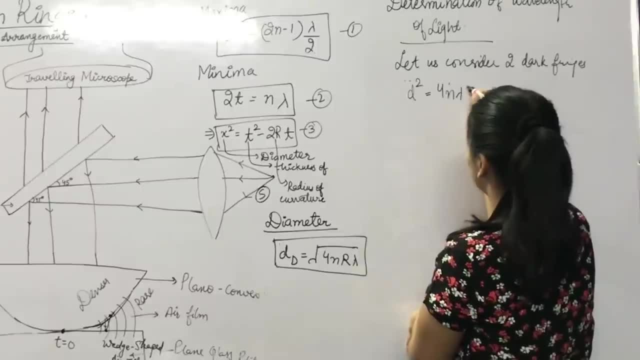 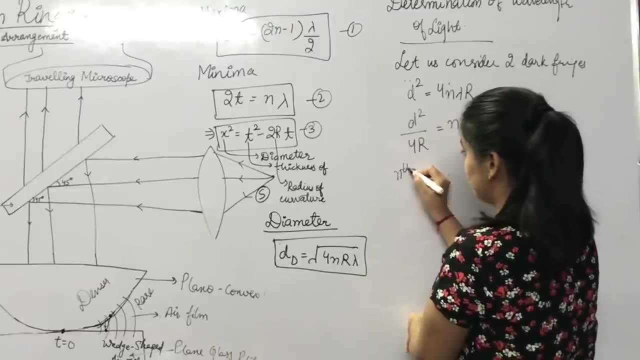 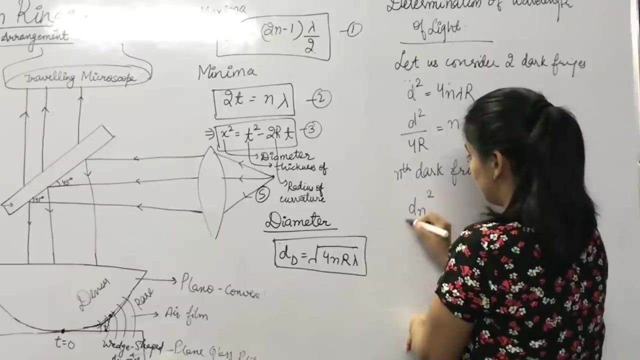 We have D square is equal to 4n lambda R. So D square upon 4R is equal to n lambda. So for nth dark fringe we have: Dn square upon 4R is equal to n lambda. Now let us take one more dark fringe. 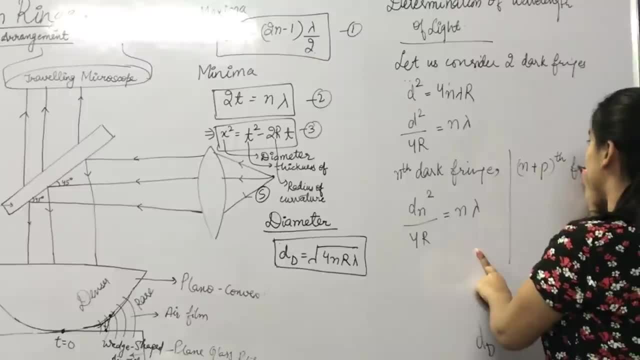 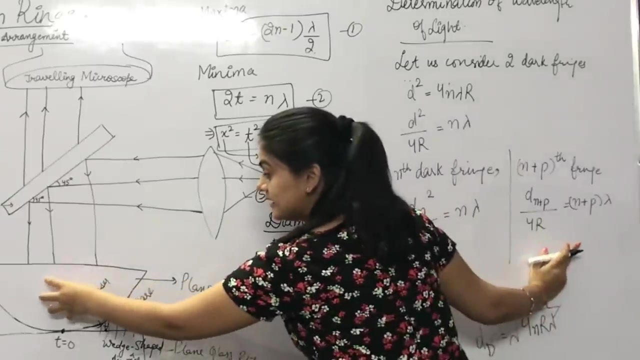 Let us consider n plus pth fringe, n plus pth fringe. So D n plus p upon 4R is equal to n plus p lambda. Radius will not change because we have the radius of curvature of this lens, So radius will not change. 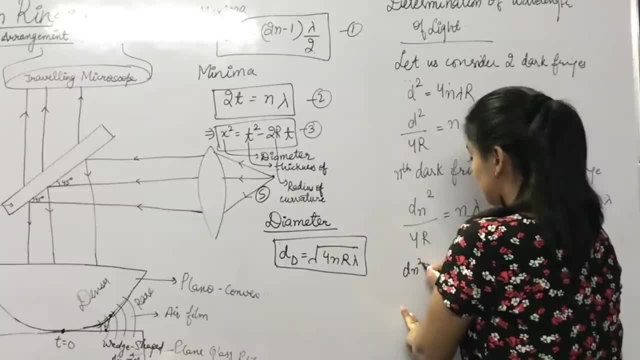 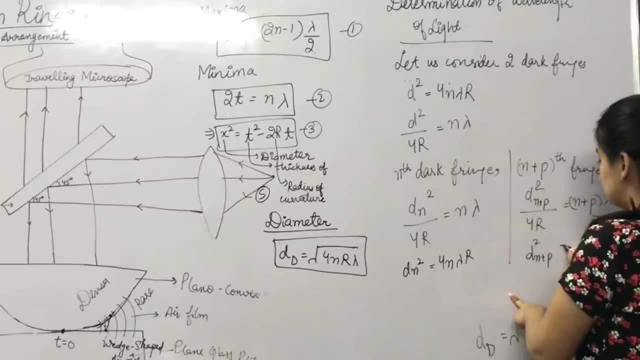 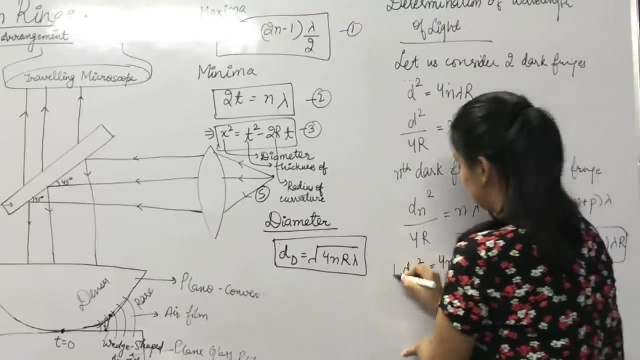 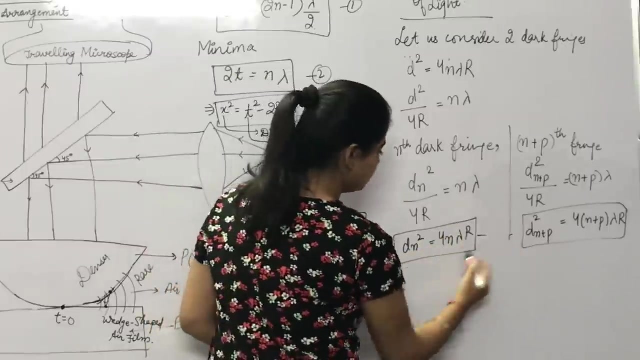 So from here we can write: Dn square is equal to 4n lambda R and Dn plus p square is equal to 4n plus p lambda R. Now we will subtract both. For determining the wavelength, we will subtract both. 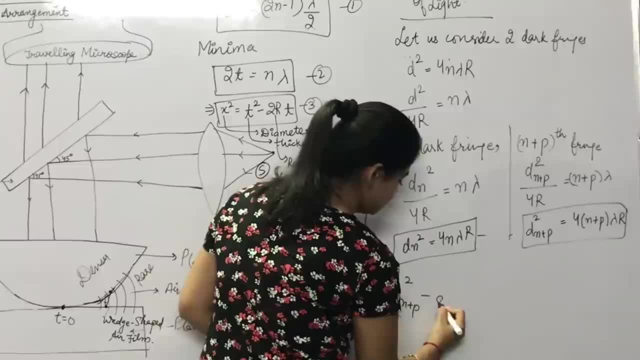 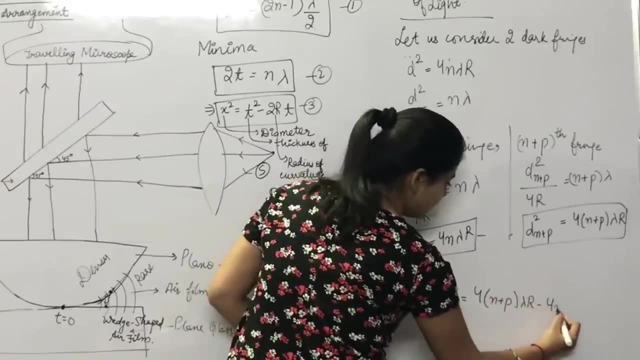 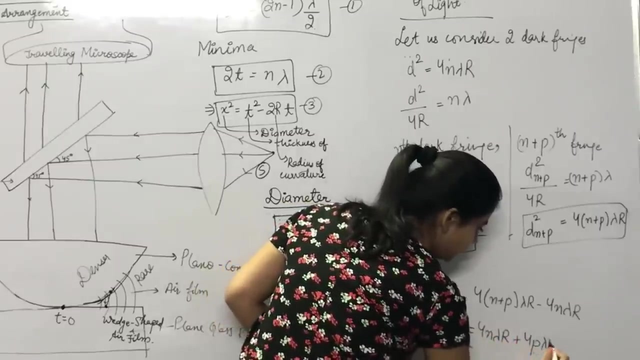 So Dn plus p square minus Dn square is equal to 4n plus p lambda R minus 4n lambda R. Open the brackets. 4n lambda R plus 4p lambda R minus 4n lambda R. 4n lambda R. cancels. 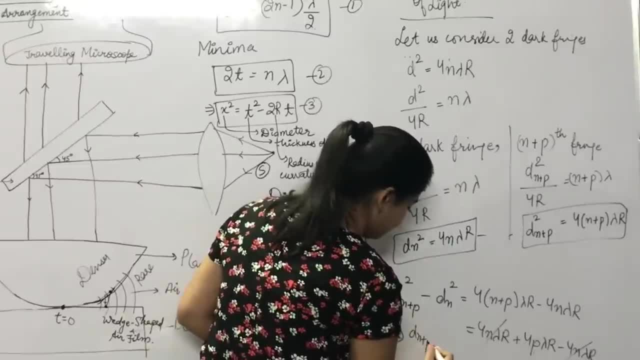 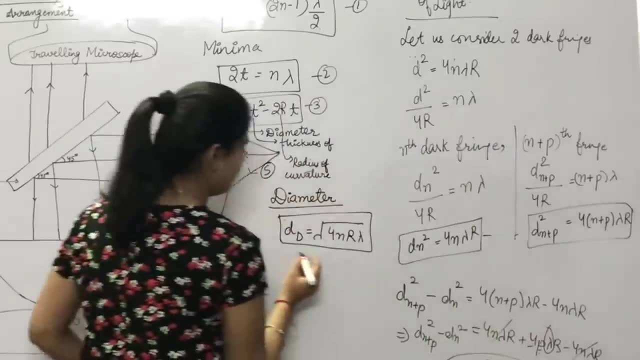 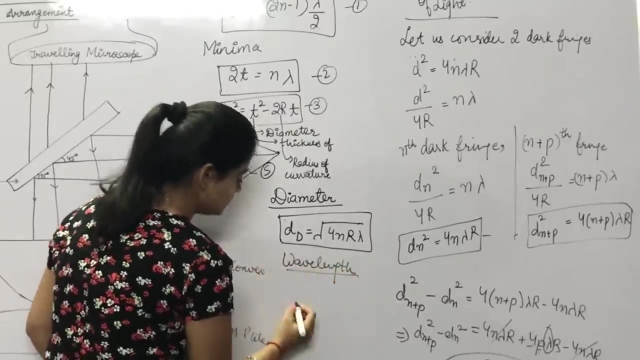 4n, lambda, R. So we get Dn plus p square, minus Dn square. From here we have to find the formula of wavelength. So we have got one more equation here. Wavelength of the light from the light source is given by lambda is equal to: 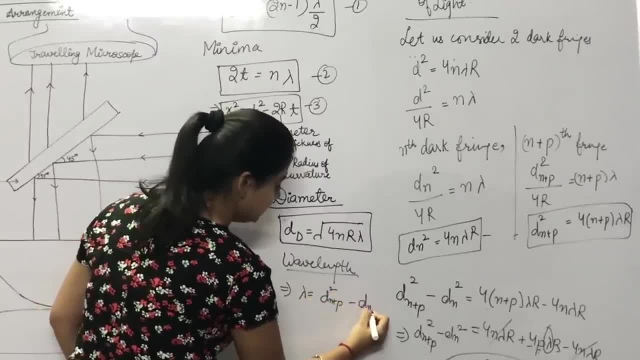 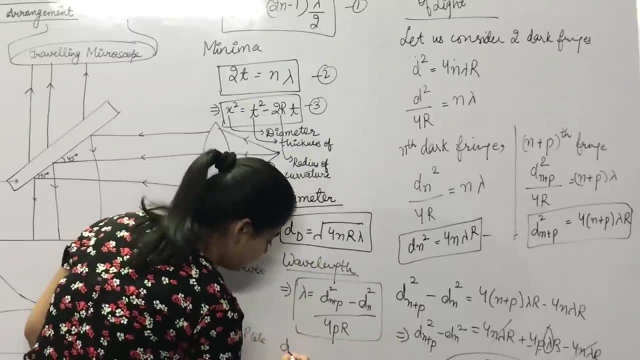 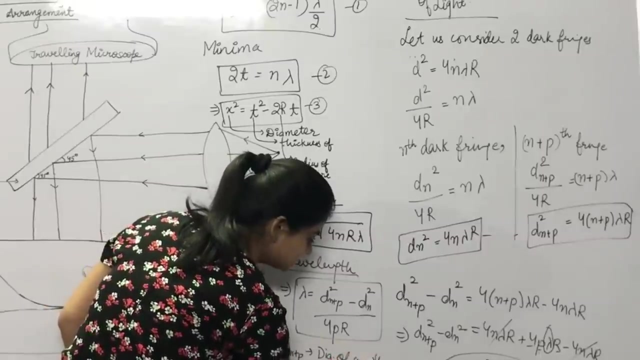 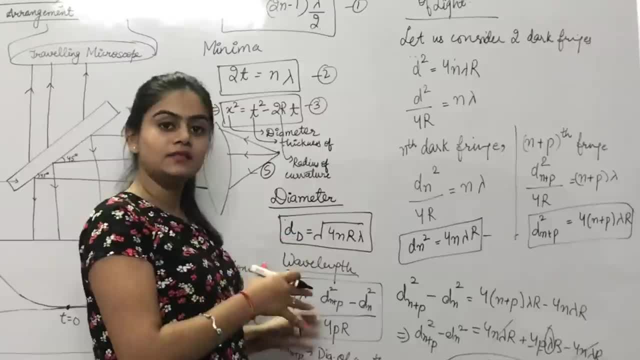 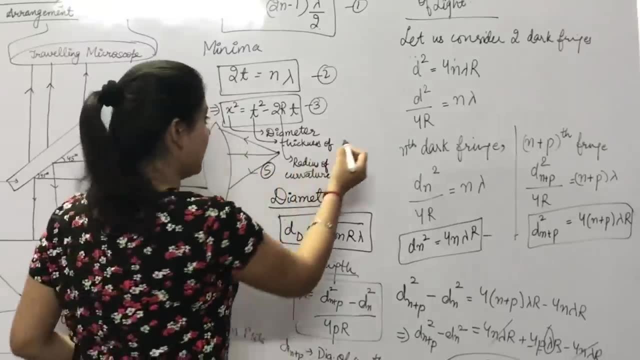 dn is the diameter of nth dark fringe. dn is the diameter of nth dark fringe, p is the difference between two fringes. How many fringes are there now? So I am taking one fringe over here, Then after p fringes, I am taking one more dark fringe. 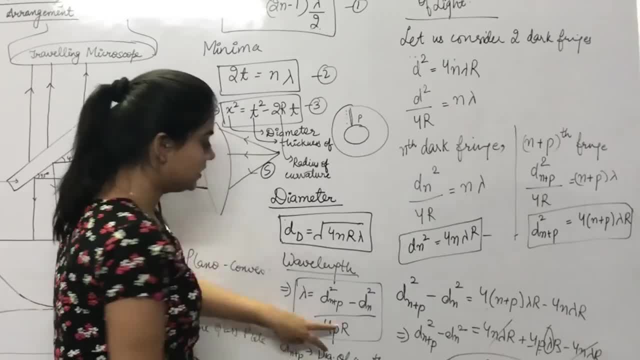 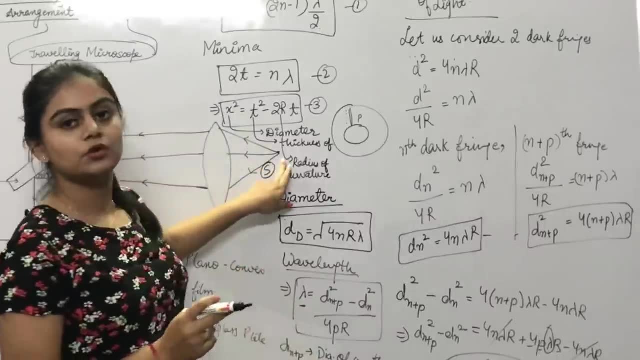 This is the difference p. So p is the difference between two fringes and r is the radius of curvature. This gives the formula for wavelength of the light from the monochromatic light source or whatever source we are taking, If we take white light source and white light source.